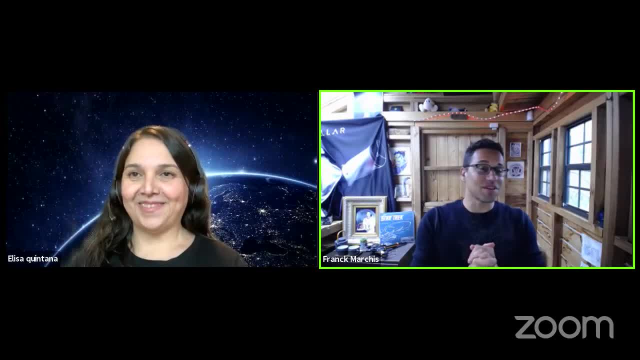 Okay, so this is a very interesting new project and to talk about this project called the Pandora Mission, we invited Elisa Quintana. Hi Elisa, how are you, Elisa Quintana? Good, thank you for having me. Where are you located, Elisa? 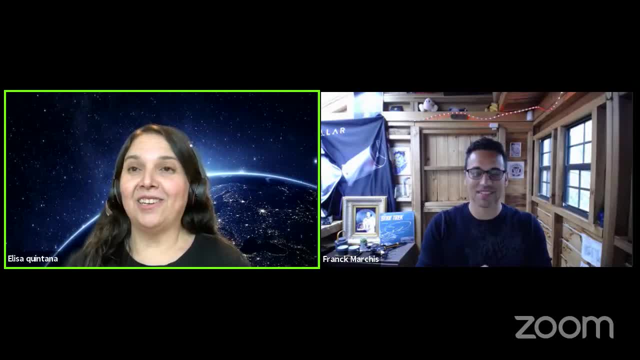 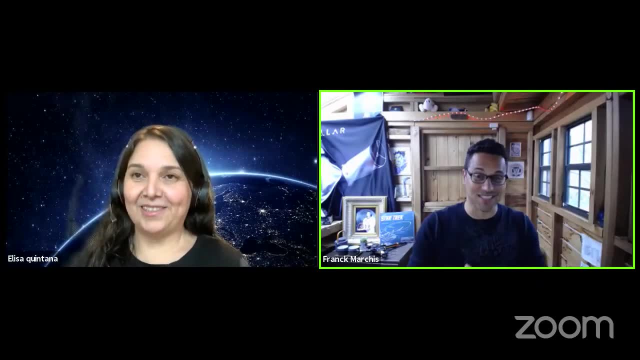 Elisa Quintana. I'm currently in Maryland. I work at NASA Goddard Space Flight Center, so the other side of the coast, Yes, so I wanted to mention that Elisa is an Astrophysicist at the NASA Goddard Space Center. 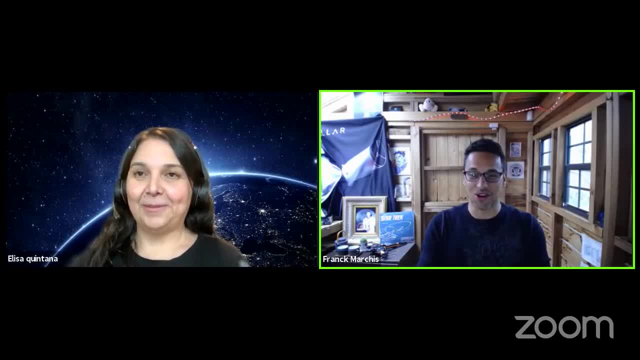 and she's also the principal investigator of the Pandora mission. She's well known from us because she worked in the past on the Kepler mission at NASA Ames, and she was also a SETI Institute employee And then she decided to move to the East Coast because she loves snow and cold weather, right. 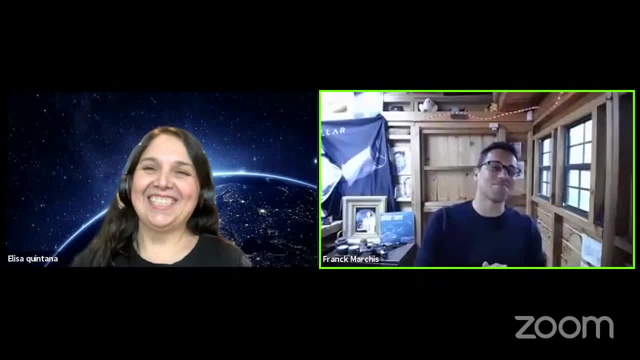 Yeah, that's right, Welcome back. We're very happy to have you here, So if you are watching us, please tell us where you're watching us from. We are going to have a conversation as usual with Elisa to talk about the mission. 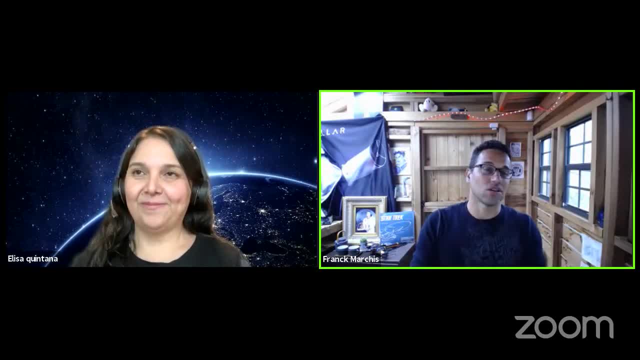 and what's the goal of this mission. And if you have some questions and you want us to address some specific point, we are listening to you. we are watching you and reading those chats. In fact, I am not doing it, Bess is watching it in the back with Rebecca and Jasmine. 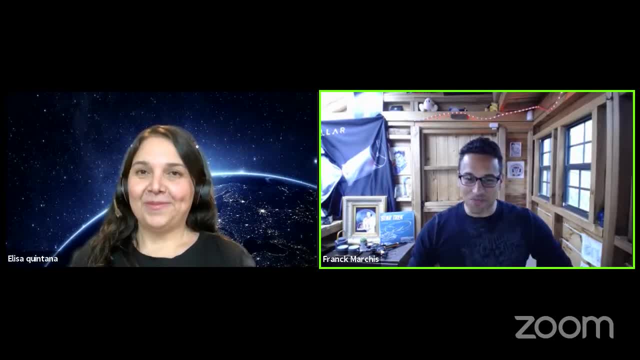 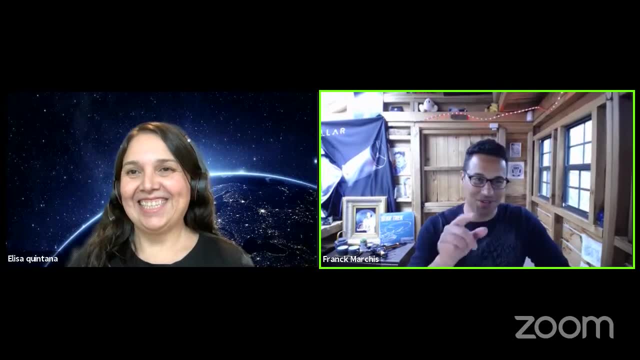 So thank you very much, everybody for taking care of that. So Thank you. So what is Pandora? This is an interesting name. first of all, Maybe we're going to talk about that, But tell us about this mission exactly. 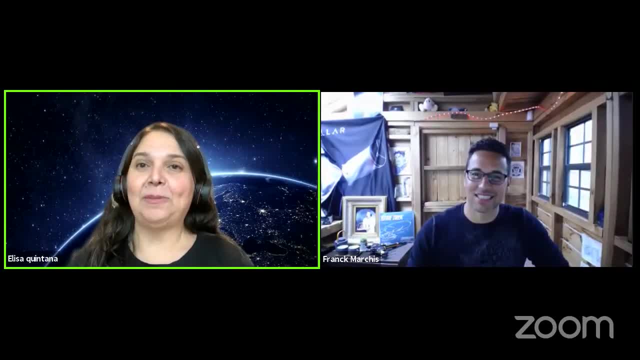 Sure. So Pandora is a small set. This is a small platform mission. It is designed to look at exoplanets, which are planets that orbit distant stars and probe their atmospheres, see if we can look at the makeup of their atmospheres. 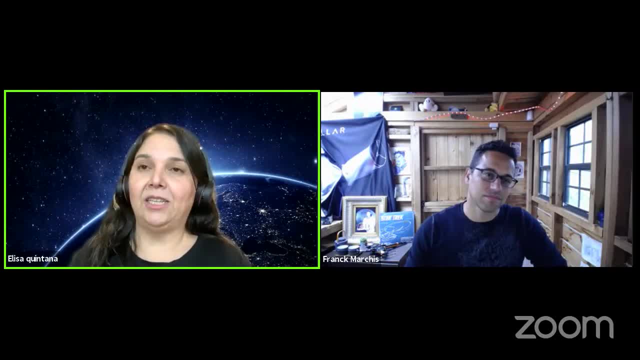 We are also. We are also designing the mission to, just as importantly, look at the exoplanet host stars, So the stars themselves, because we know that small stars can be really active and we're trying to see how much this activity influences our observations. 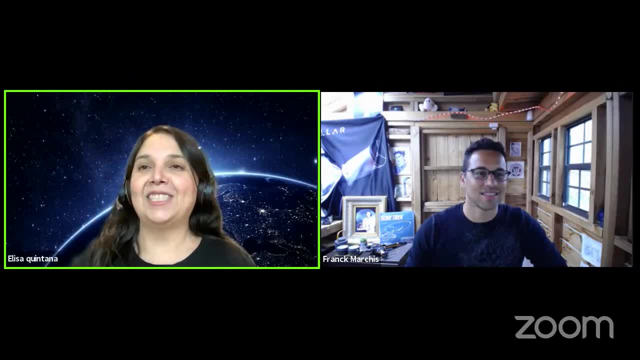 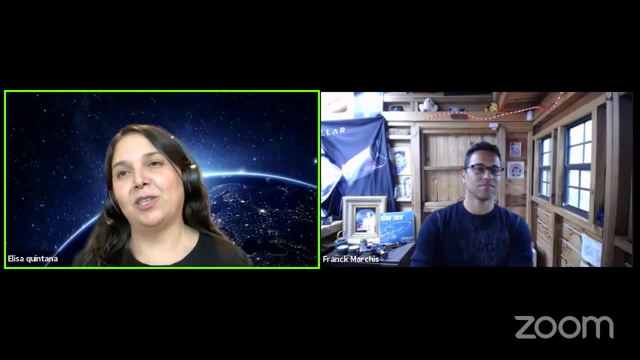 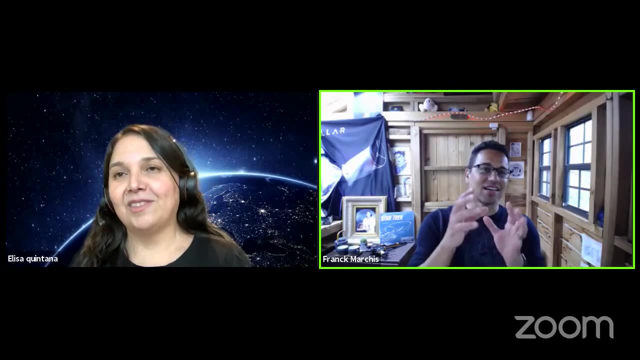 and how robust our measurements can be, And so it's a nice. you know, these small sets are nice platforms to complement these upcoming big missions, like the James Webb Space Telescope, to really maximize the science from those. Yeah. So maybe we should mention that NASA has divided those missions in different categories. 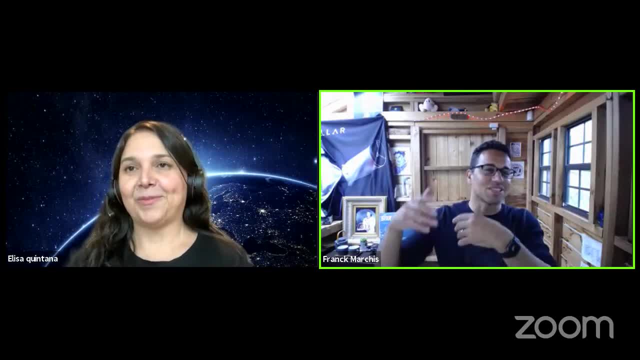 There is the Discovery mission, There is the Flagship mission And this is a kind of a new program called the Pioneers program. So we say small set. We're talking about what? Something big like that or the size of a house. 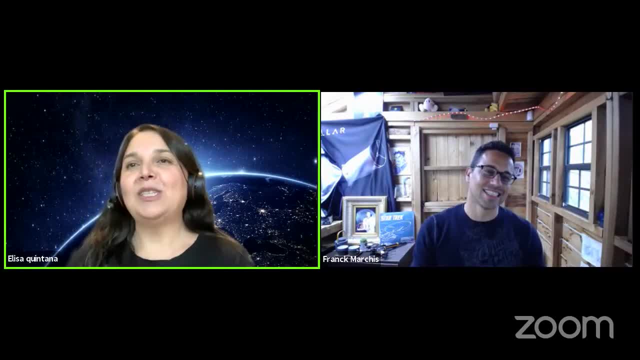 What is a small set? Yeah, So a small set is sort of in between a CubeSat And you know, as you said, NASA has a bunch of different kind of levels. They are given different funding caps And so if you think of CubeSats have been around a really long time. 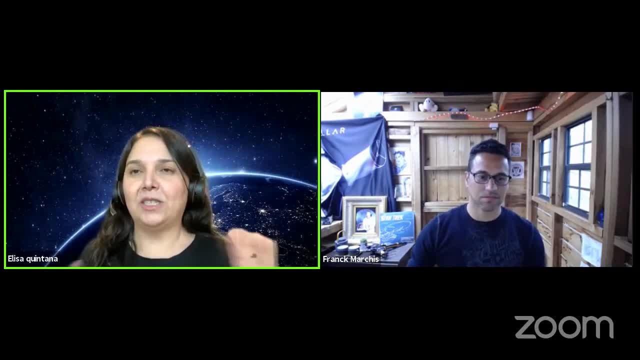 you know those are great platforms for universities and their students to work on those, And those come in volumes which they call kind of cubic units, And so you can have like a CubeSat this small, or you can have it the size of a cereal box. 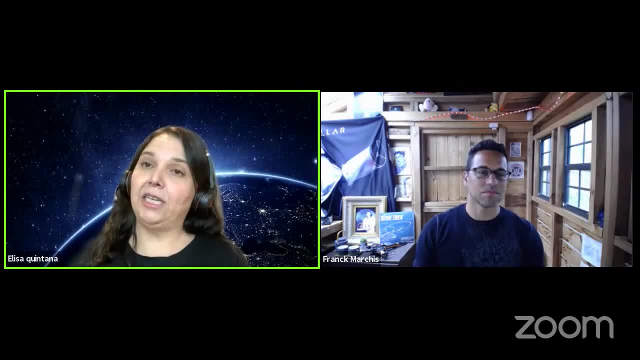 And there weren't a whole bunch of opportunities, you know, to design missions that were larger than that, but smaller than explorer class missions, such as the test mission or even something larger like you know, Kepler or even Hubble. So NASA is really interested in seeing what kind of astrophysics we can do with something. 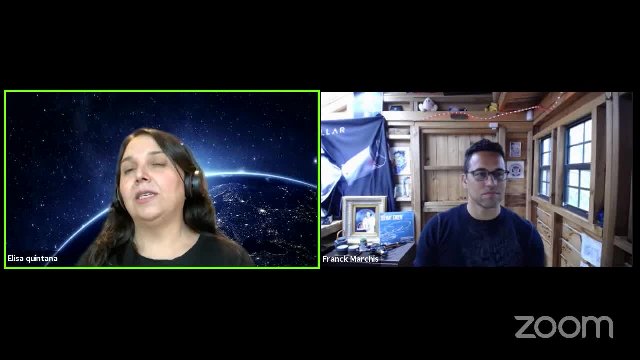 you know the small set regime. So the Pioneers is a program that's a $20 million cost, you know, and it's really interesting. It's a big program And so we have a lot of different kinds of missions. 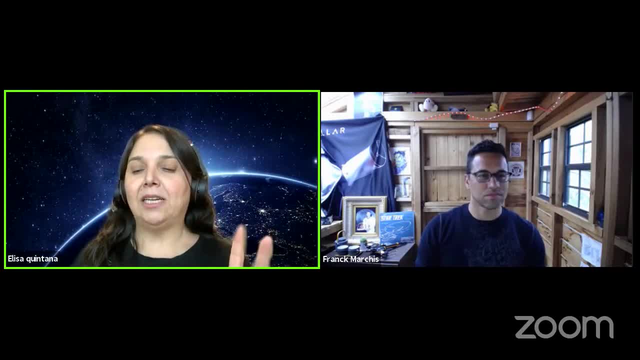 but they're not, they're not really the most, you know, the most advanced total for these missions. And so what we have, it's not so set in terms of volume like the CubeSats, but it's still, you know, relatively small. 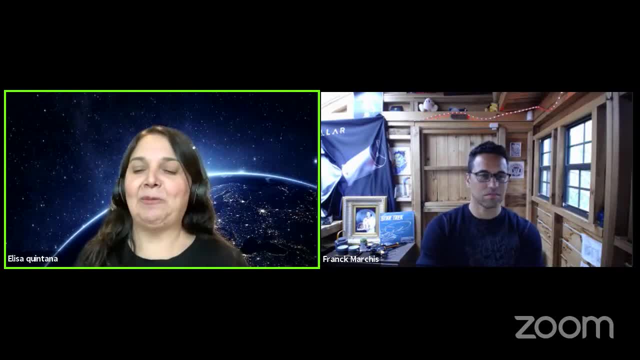 And then we designed this mission and we and then we ended up on a ride share for a larger mission. So we put everything together and then we kind of wait and we'll tag, tag along to go on, you know, into orbit with when something bigger goes up. 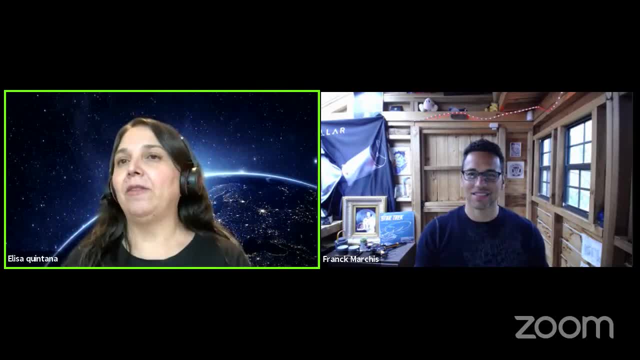 So it is a new class for astrophysics. For astrophysics, for sure, We have lots and lots of, you know, all kinds of sizes for Earth science and planetary science, But for astrophysics, you know, we're trying to really understand what can we do with this kind of size and scope? 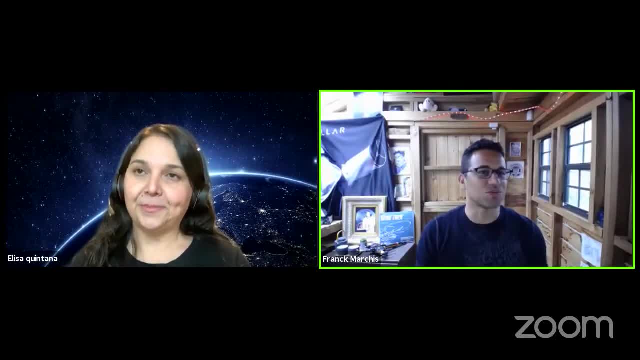 So this is a low-cost mission in 20 million compared to all the other missions, Like Discovery is 450 million, if I remember, for instance in planetary science. So it's 20 million is to cover what: The launch, the operation, the data processing. 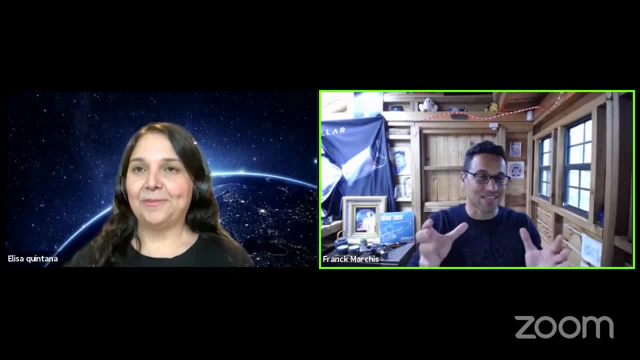 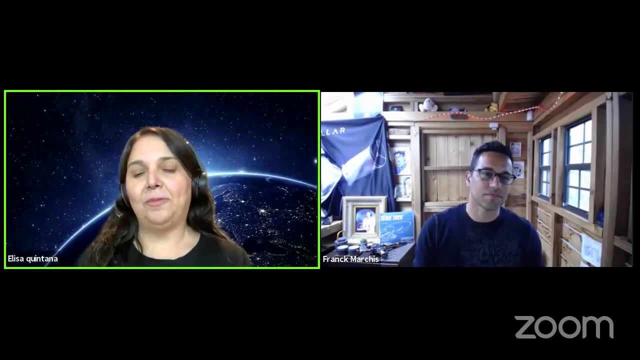 What is the mission itself? It's not only the satellite right, It's everything else. It's everything except for launch. So NASA covers the launch, But it's everything from engineering to design the mission, to build it to. you know, it's also a five-year program. 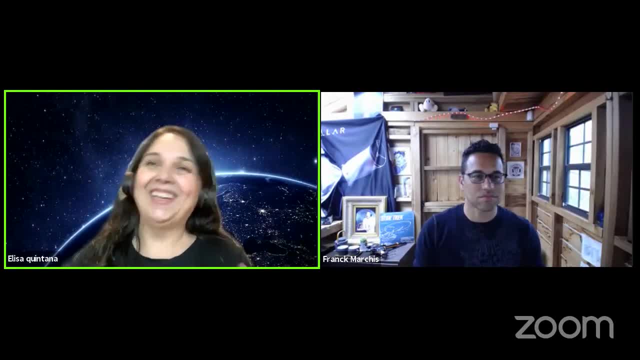 So, unlike bigger missions which can take, you know, decades, it's a five-year mission from you know the time We start and the time we launch the mission, fly the mission, get the data, write papers, everything. 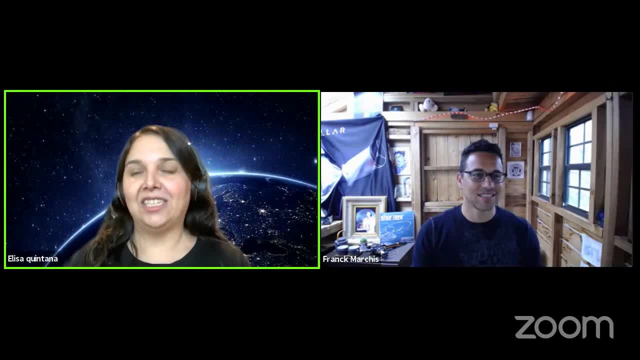 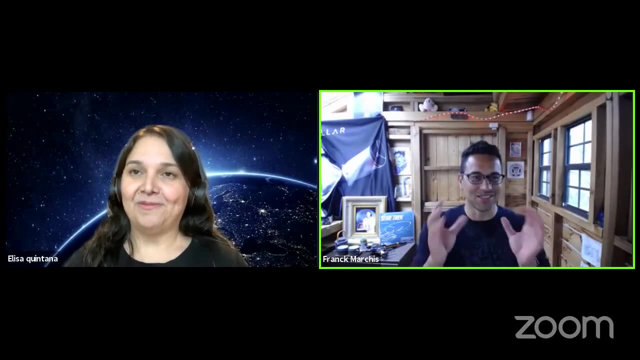 So one nice thing is: you know it's a challenging timeline, for sure, But it is nice to have to know that you can do something within five years. Yeah, it's kind of the startup of the mission. You do everything very quickly and launch it, operate it, observe it. 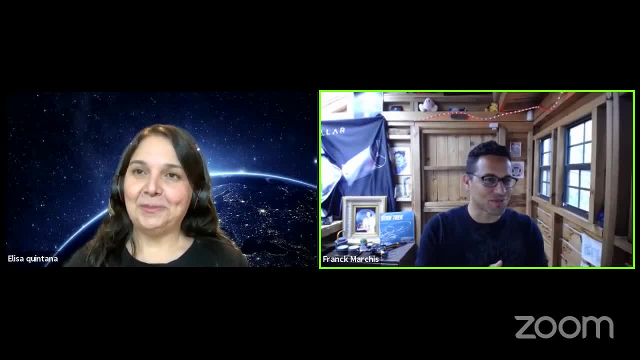 So what's your role in the mission? Yeah, I mean it's a very complex program. I say principal investigator, but for most people we don't really know what it means. So are you building yourself the satellites in the lab or what's the role? 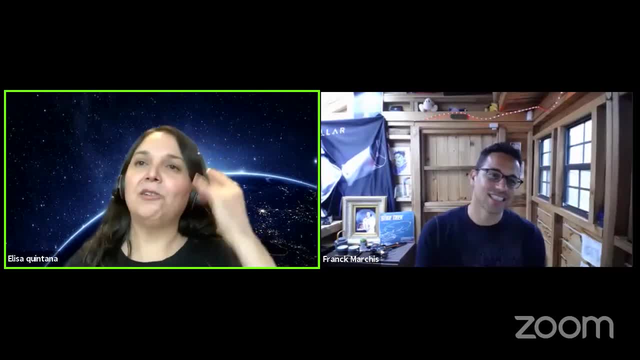 And maybe tell us a bit who is building the satellite as well. Yeah, sure, So principal investigator is basically the person that leads the mission. You know we- I'm not in the lab myself, you know, I'm coordinating everything. 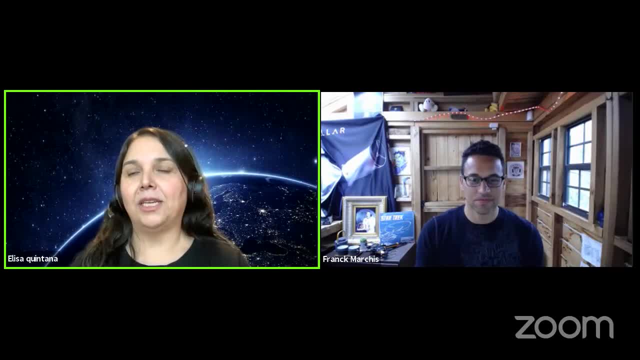 And so every mission has a principal investigator, Except for the big flagships. I guess it's structured a little bit differently, but we have partnered with Livermore Lawrence Livermore national lab, which is in your neck of the woods. They have a fantastic group that is doing everything from the optics to procurement. 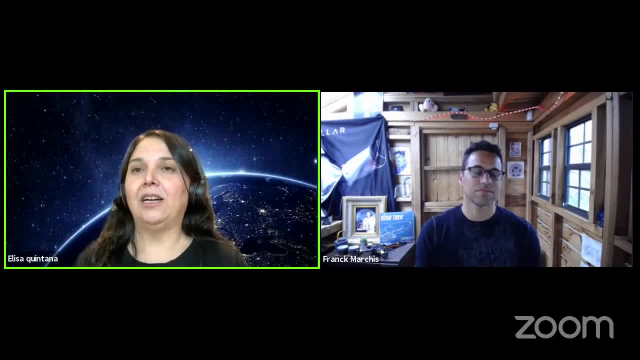 you know, buying everything we need, the engineering. they're also managing the program And so it's a little bit of a, a unique kind of experiment for us at Gartner Goddard, because typically NASA Goddard manages and builds a lot of stuff. and then the principal- 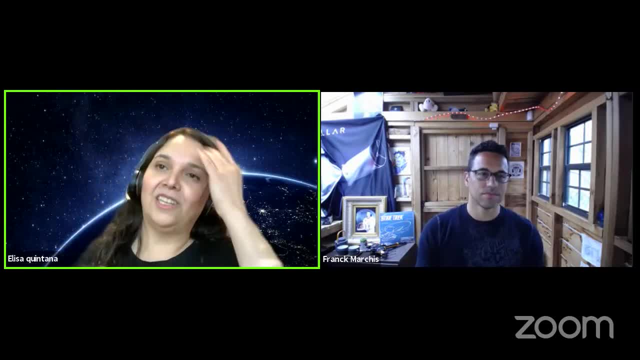 investigator, you know, can sometimes be at a university or external, and so at this time we're trying, we're doing a switch to see how this works. and you know, with these classes it's, you know, when you try to launch something on a lower budget, you it is, they are higher risk. so all of these you 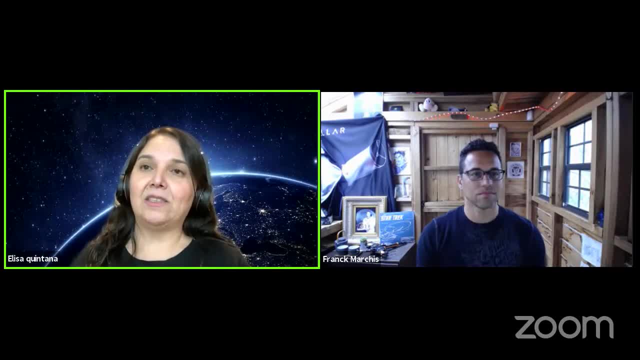 know smaller missions are higher risk, high reward. that's something NASA's trying to do more of: to see what kind of you know science we can get and you know with, without spending so much money on so much testing and so much oversight. that's just build and see what happens. but we have a great 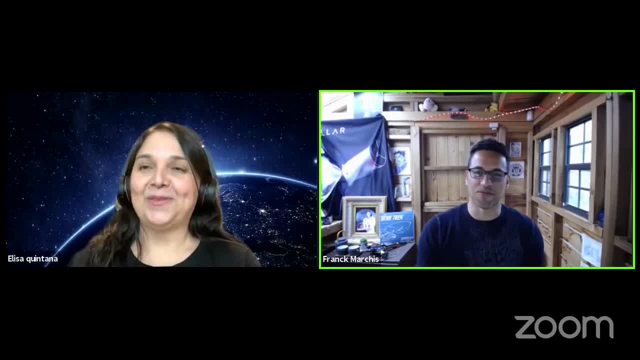 team, launch it and operate it and hopefully get some good data. so that's a good transition, in fact. but before talking about the transition, let me tell you that we have people watching us from Canada, Germany, Ireland, Denmark, Decatur, Indiana, Netherlands. 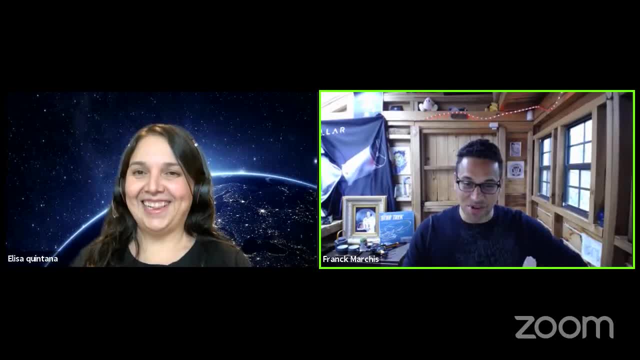 San Francisco, myself and other people apparently Severin in Florida, North Elman in England, Sintra in Portugal, Salingrove in Pennsylvania, Colombia, Montreal, Ecuador, Philippines, Laos, Pakistan and Toronto, Canada. So you're welcome. we are talking about the Pandora mission. 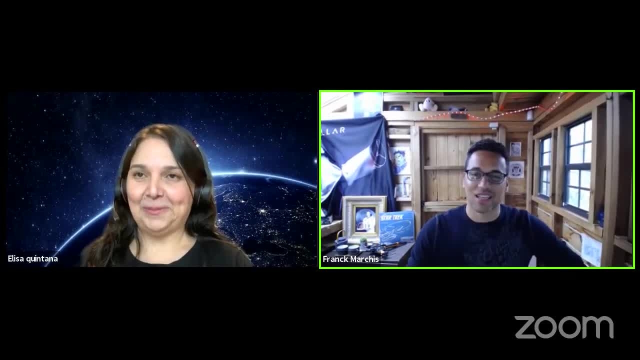 a small sat, a small satellite that could detect and characterize the atmosphere of exoplanets and both the Earth and the sun. so you have a really important mission. you're going to need to do long-term research in order to get to a more authoritative solution. So what is the scientific? 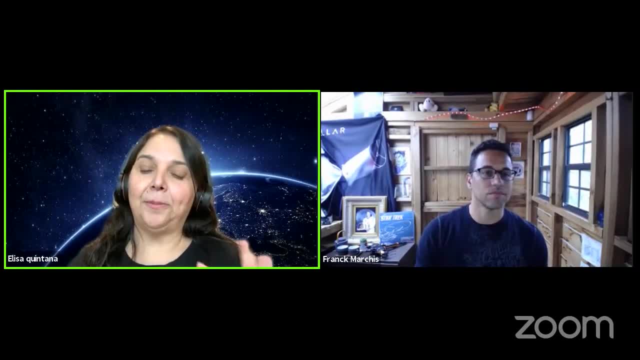 purpose of Pandora and what kind of information you're expecting to get from this mission. Sure, so NASA has a roadmap and, you know, driven by some of these big science questions, how common are other Earth-like planets? are there life on other planets? You know these questions, driven by the SETI Institute as well, and so you know, we have the Kepler mission, which will be in 10 and 15 years from now. 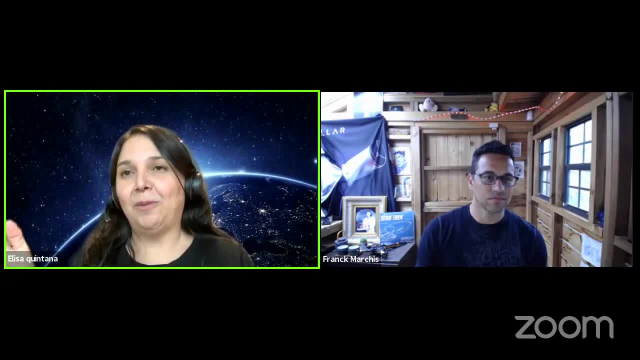 which launched in 2009 and found that planets are common, with thousands of thousands planets known. Currently, the TESS mission is operating and finding planets that are closer to us that we can study in further detail, And then the next step is James Webb, which has a 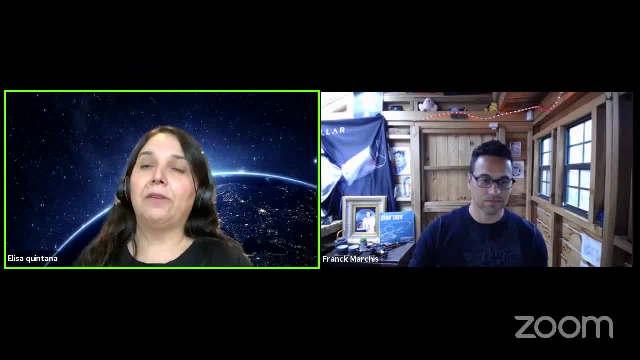 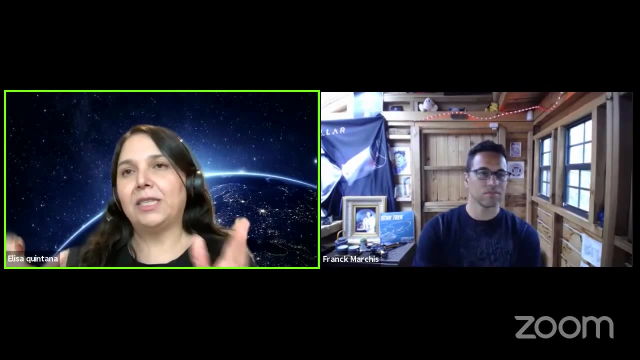 scheduled launch for October. James Webb is going to have capabilities to really look at exoplanet atmospheres to unprecedented detail, So we can really learn a lot of information on many planets. Do they have atmospheres like Earth? Are they more puffy like Neptune? And? 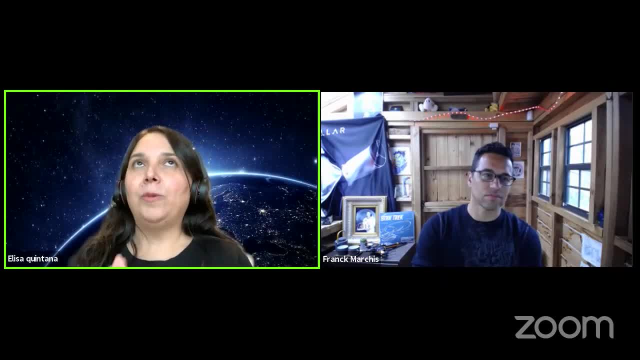 kind of rewrite the textbooks for that. And so while we are building these missions and we're gaining new technology to probe further and further, and our measurements require so much precision, now we kind of have to take into account a lot of factors that we typically could. 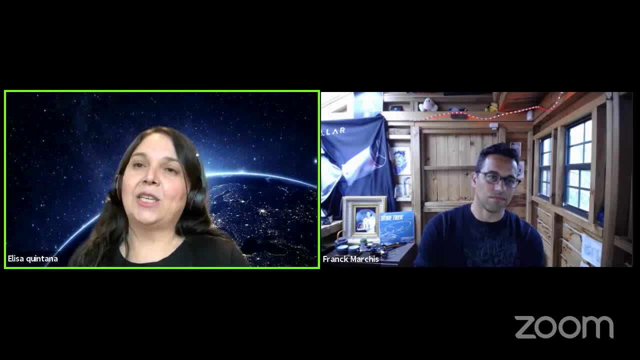 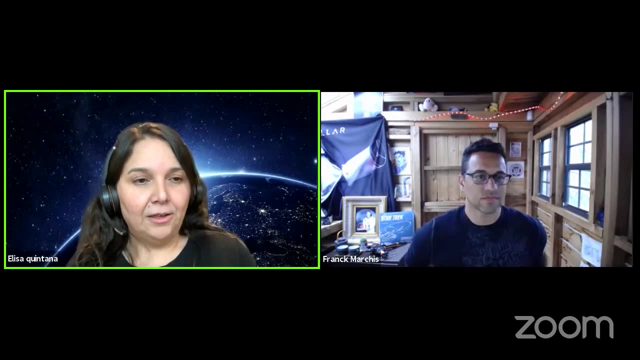 you know, just kind of ignore. And so one of them is stellar activity. So we know that stars are active. We see that on the, on the sun, You see lots of flares and star spots, And I wanted to show this quick graphic, Put it on play. I'll just leave this up for a 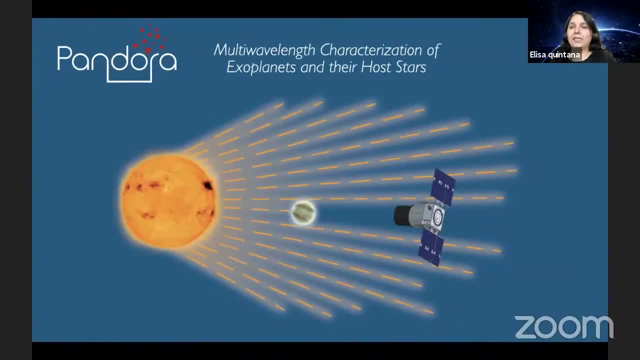 moment. So one of the ways that James Webb is going to characterize atmospheres is by looking at exoplanets when they transit their star, And so, essentially, when a planet's crossing in front of a star, starlight filters through the planet's atmosphere And, depending on what atoms and 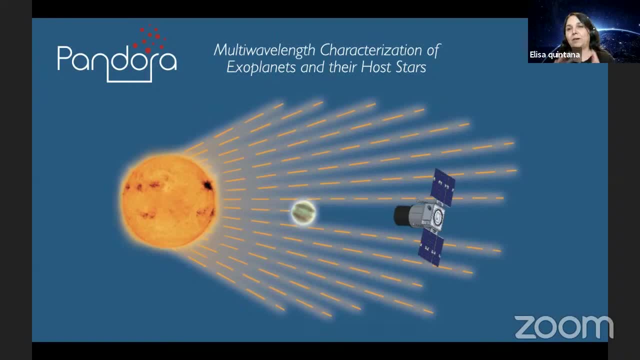 molecules are in those atmospheres and you know what wavelengths of light they absorb. we can learn a lot about what they're composed of. So that's what we're going to do here. So just to they're composed of. And so this whole technique only works if you assume that the light coming 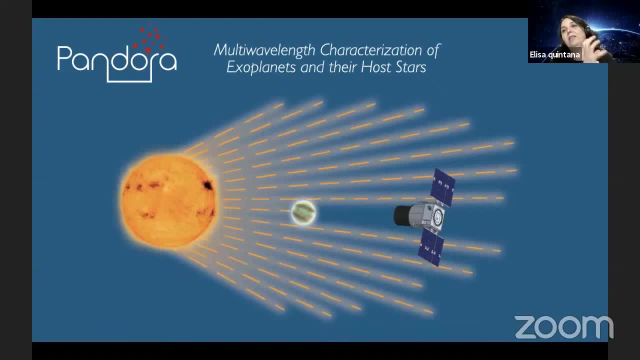 from the stars is uniform and constant, because you're basically looking at the planet before transit and during transit and subtracting at the star to get the planet's atmosphere. But now that we're looking at really really fine detail, we do have to take into consideration. 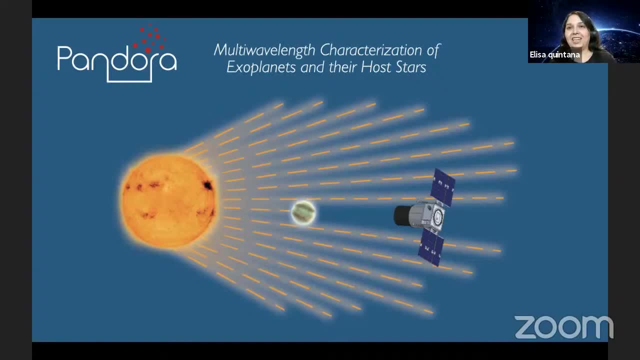 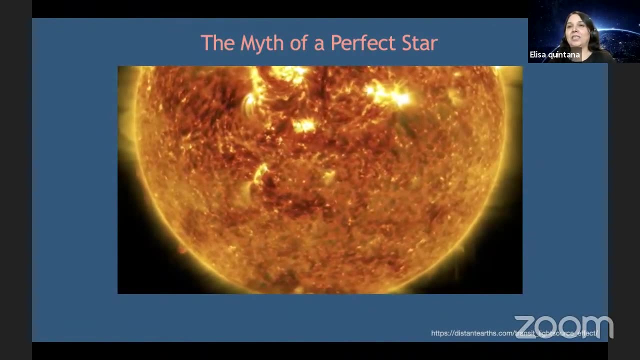 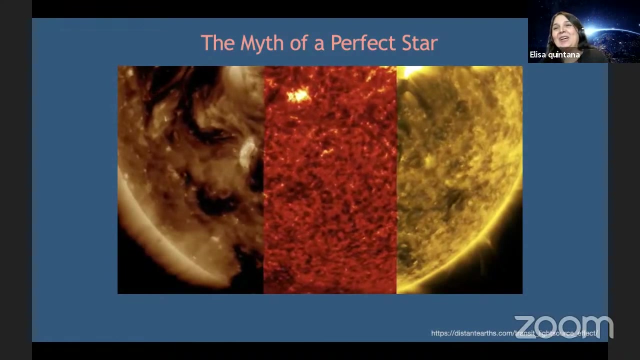 stellar activity and that's why we built Pandora. And I just wanted to show this movie- and it's my last slide just to kind of illustrate. So this is from the Solar Mission SDO that shows Mercury transit. You can kind of see it somewhere along there, But this really 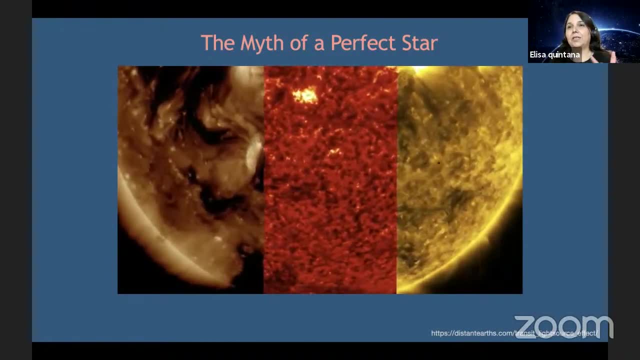 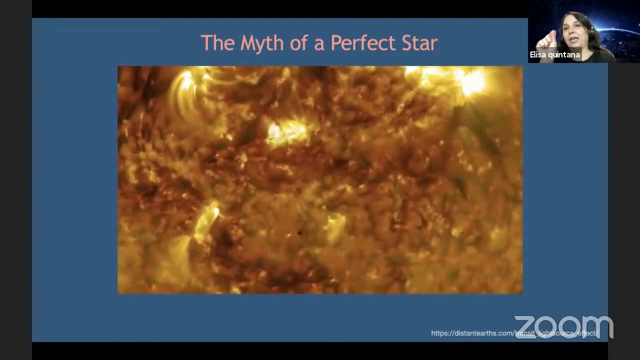 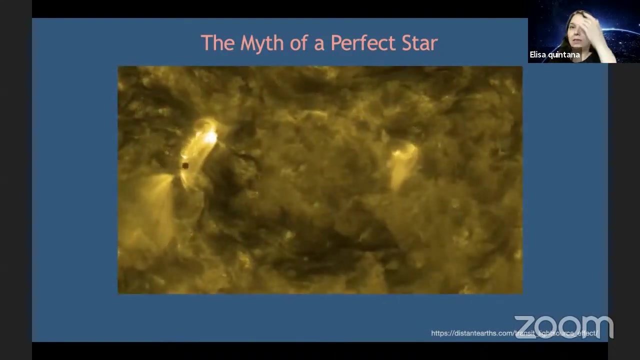 shows, even for the sun, which is a quiet star, that there's still so much activity. And so, if you think about, we're trying to measure this tiny atmosphere around this planet, but there's so much variations in light coming through that essentially can contaminate the atmosphere. 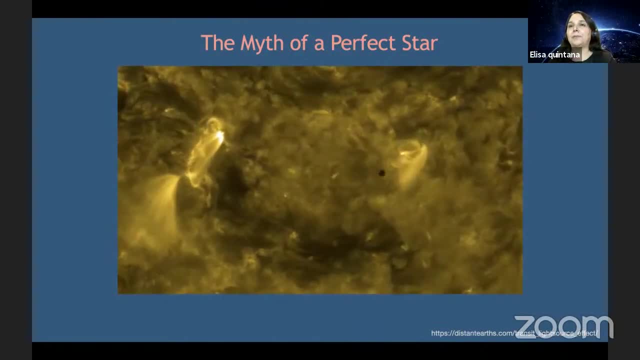 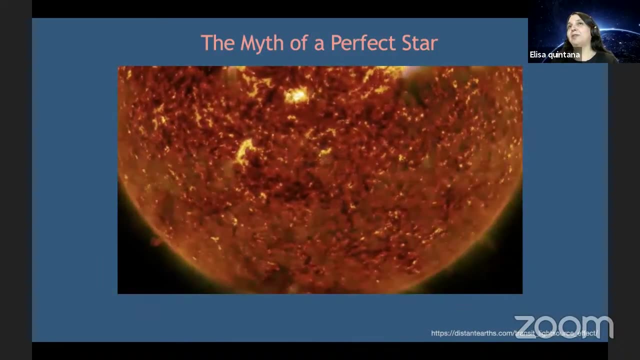 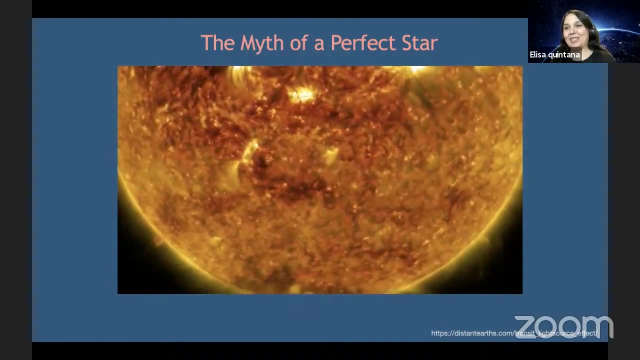 of the planet. This is a sort of a new problem that a lot of people have been focusing on lately, because when we observe planets with James Webb and say we discover water in the atmosphere of a new planet, we want to make sure it's water in the atmosphere of that exoplanet and it's not. 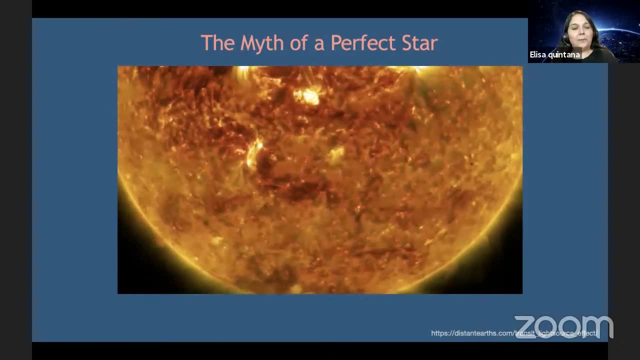 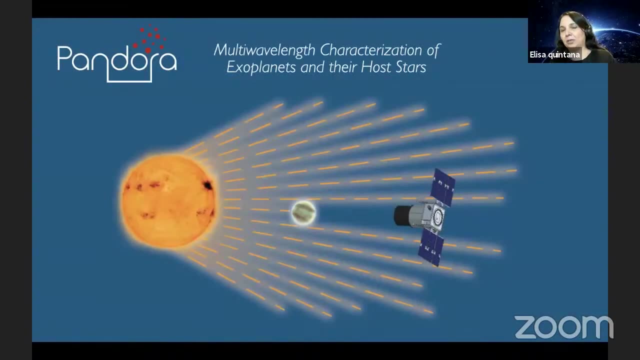 variation from the star that's contaminating it. So that's what Pandora is doing. The previous slide showed. you know, it's using the same technique that James Webb is going to be doing, But whereas and the same technique that Hubble has used to probe the 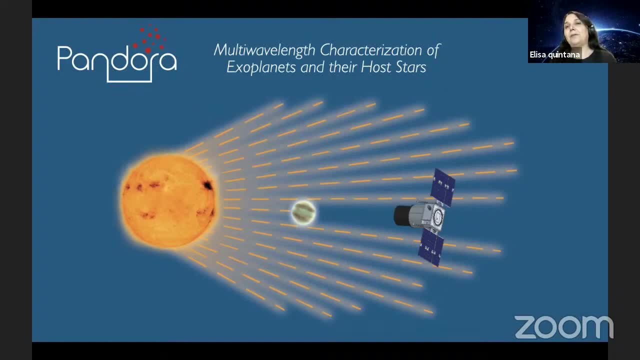 atmospheres of giant-sized planets, But instead, you know, Hubble and James Webb have these precious telescope time And so they typically will just observe one transit, and you deduce, you know, information from that: What Pandora is going to do is observe these transiting exoplanets. 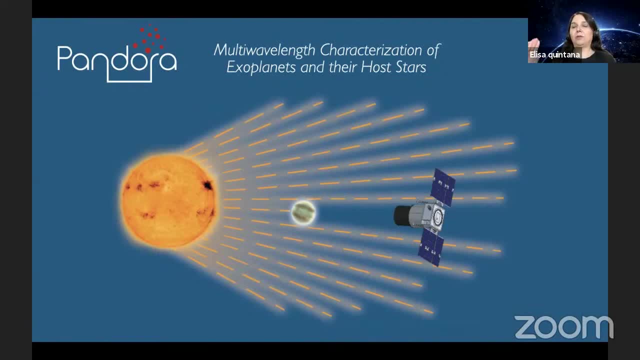 for a really long time, So for 24 hours, to see 10 transits for each exoplanet, And then by doing that you can get a lot. you can capture all of the information of what's going on with the star and see how much of an effect the stellar- you know what we call. 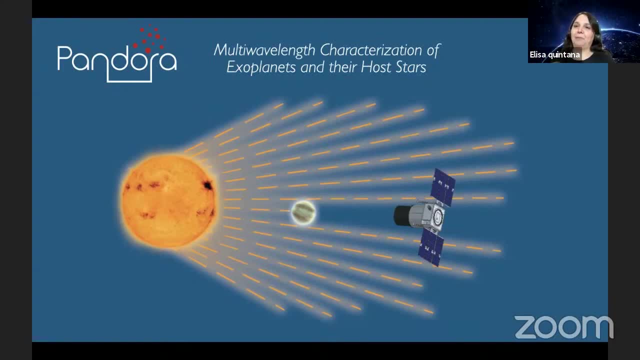 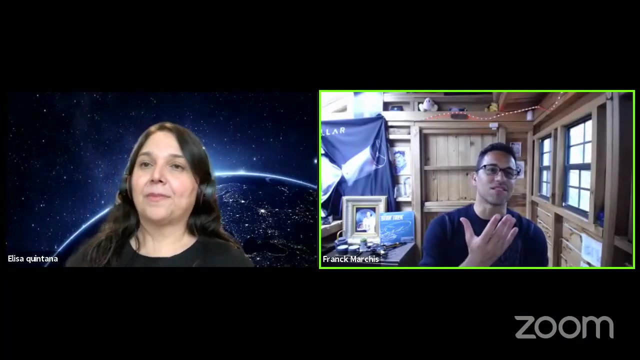 contamination is in these measurements and mitigate it. So we can have be really confident that we're finding these fantastic features in exoplanet atmospheres. So, in short, the problem we have here is that you, instead of discovering planets like Tess and 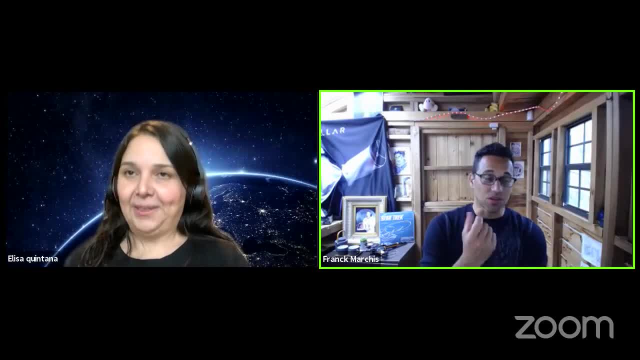 Kepler has been doing. you want to characterize the atmosphere. To characterize the atmosphere, you really truly need to know what the star which is in the background is, the type of activity the star has. So you will do multiple measurements of the transit, of the transiting exoplanets. 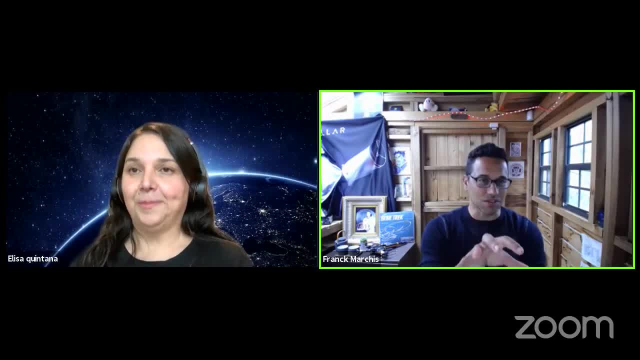 So you either average or better understand the variability of the star. So you can see the thin absorption bands relative to the presence of gas in the atmosphere and not due to the activity in the background from the star. Is that a good summary? Perfect, yes, Okay, so that's very. 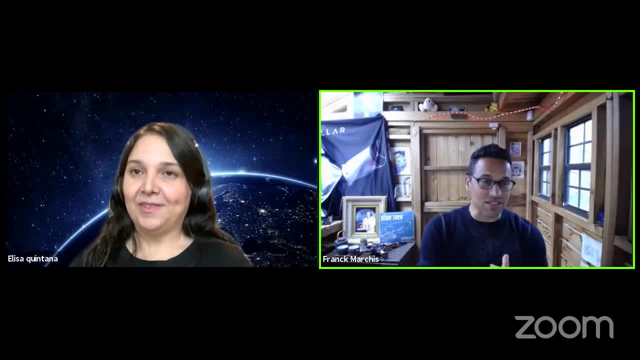 interesting and we have done that, as you say, with the Hubble Space Telescope for some candidates. We will probably do that with the JWST when it's going to be flying. What about those planets? I mean Pandora you mentioned. Pandora is a small satellite. You did mention the size of the 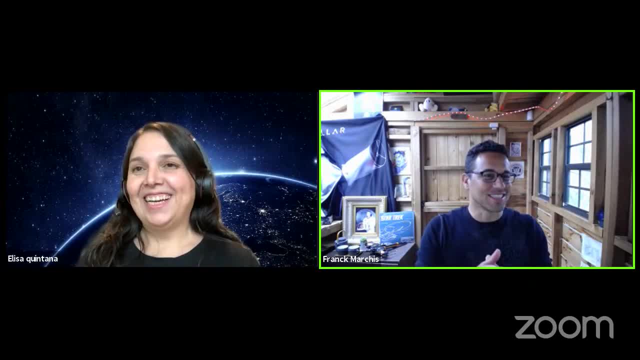 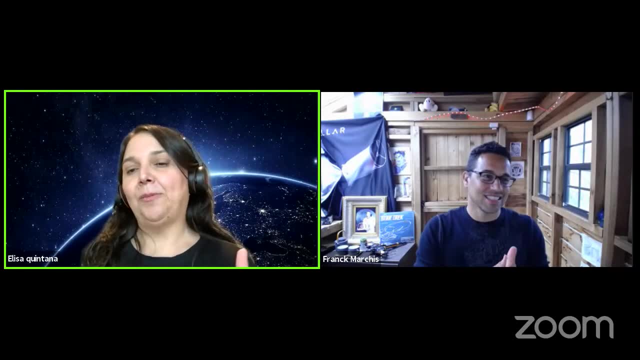 of the aperture, by the way, which is not really what people say. What is it? It is 0.45 meter telescope, and so what is unique about Pandora is that we have two detectors that will operate simultaneously, So one will be capturing visible light, So we can see variations. 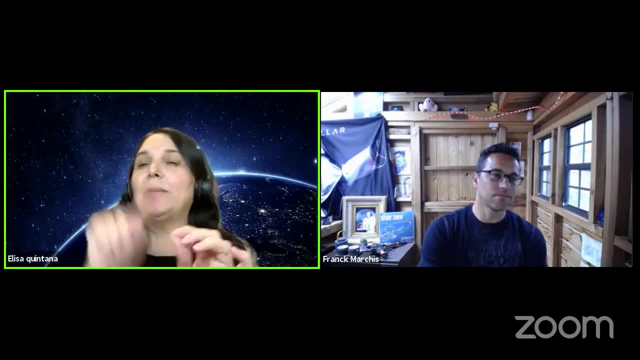 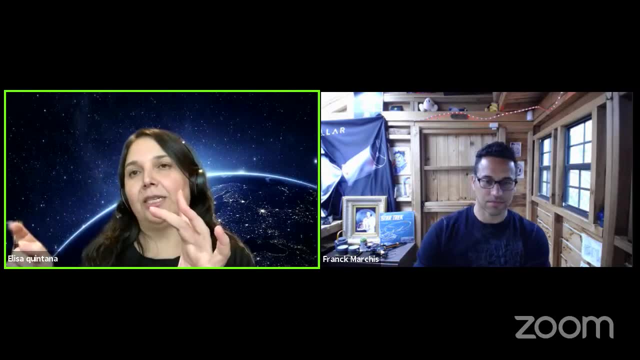 of the second telescope's, So we don't have to operate Οーο ο's. if you're using some observation detection system, You um of a star and the reason you see variations is because, uh, you're, you're basically measuring brightness over time. you know that's how we detect transits, um, but if you have star spots, 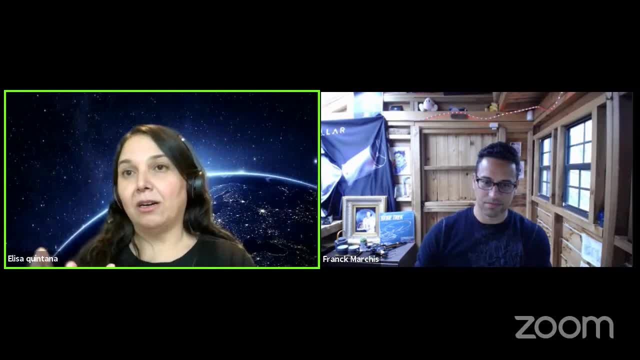 rotating in and out of view, um, some spots can be dark, some spots can be bright, and so you can track those uh star spots coming, you know, from the rotation of the star um, and then, simultaneously, we'll be taking uh spectra of of the exoplanet. so, um, by operating both of these simultaneously, 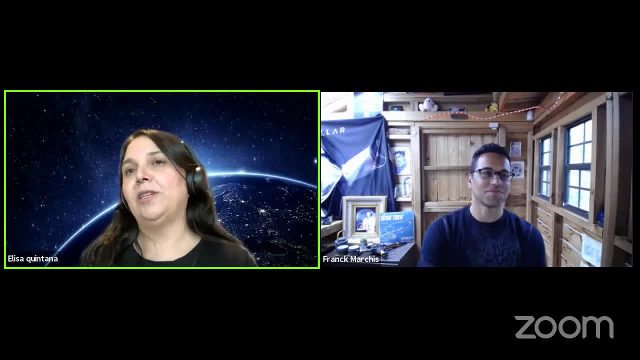 we can disentangle the star and planet signals, and so that's really what's. what's unique about pandora is is being able to observe these for a really long time, because you'll you would never get that much. tell us you won't get 120 hours of telescope time on hubble or web you know for for. 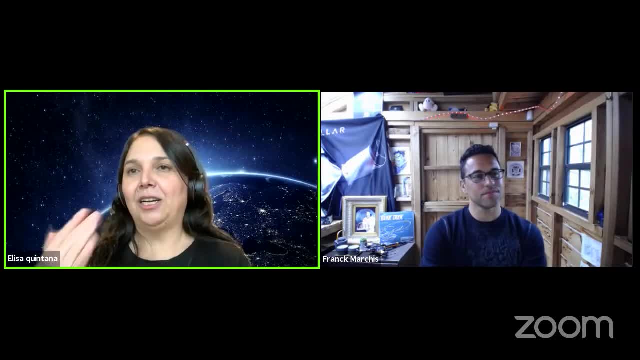 a single exoplanet, um, and and the uh, multi, broad, multi wavelength observations and, you know, for 20 million dollars, um it's. it's essentially a calibration mission. you know, we are trying to understand this, this effect, and we will be able to, um, you know, once we can disentangle these star and planet signals and remove the stellar effects. 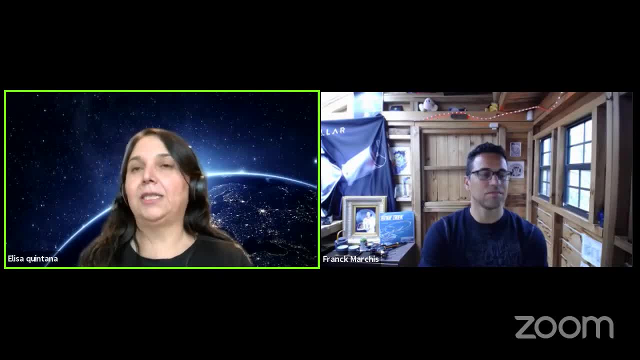 uh, we'll be sensitive to water in the atmosphere. we can see if it's a hydrogen dominated atmosphere. um, pandora's goal isn't to do these ultra high precision measures, but we will be able to do these extra measurements of the exoplanets, like that's what james webb will. 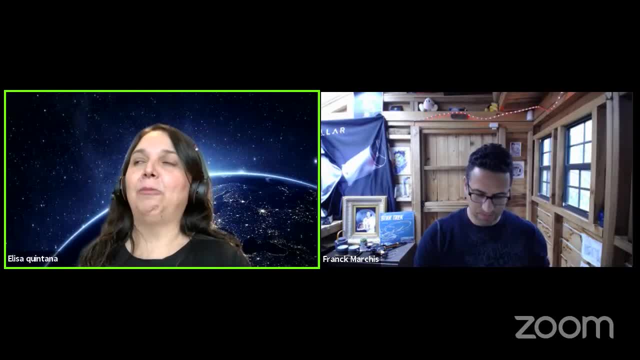 do like we're not. we won't compete with eight billion dollars in in the james webb space telescope, but we will uh be able to um provide this calibration to get the best results from james webb. so so these um small sats, and even cube sats and balloons, and all of these smaller missions are a. 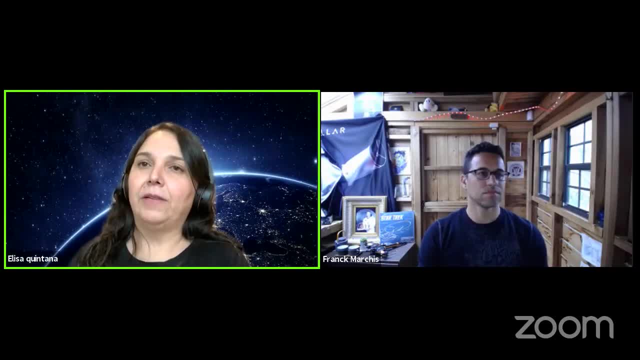 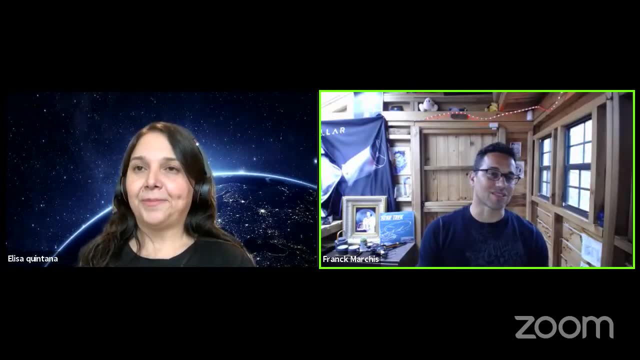 great opportunity to do things to complement these flagship missions. well, let people need to understand that those flagship missions are being shared by thousands of faster astronomers and- uh, most of them are extra galactic people. they observe galaxies, have bridge chief very high, so super far, super faint, so they observe for hours and hours. so 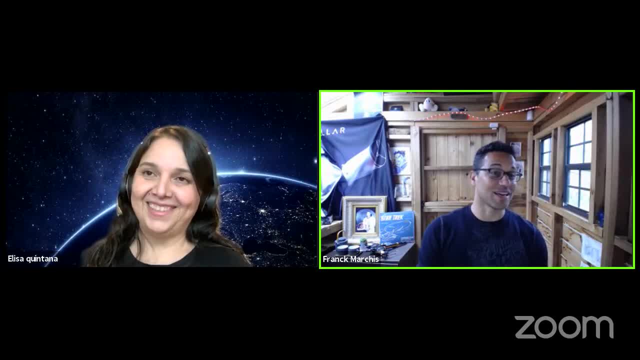 people like us, exoplanetary scientists or planetary scientists. even we don't have a lot of time. we just share like a few percent of the telescope of the gwst time, And what you don't want is to waste a lot of time doing calibration instead of doing real scientific analysis. 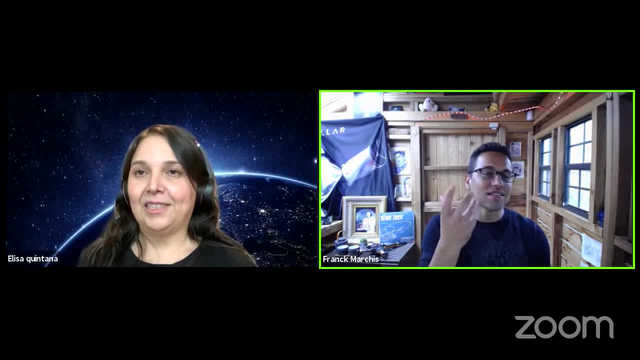 So this mission will basically calibrate somehow the activity of the star versus the activity, the presence of molecules, interesting molecules in the planet. So which planet are we talking about here? Did you select them already, or are you waiting for tests to define them? 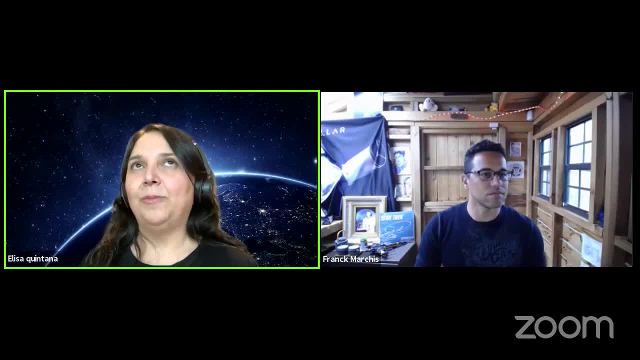 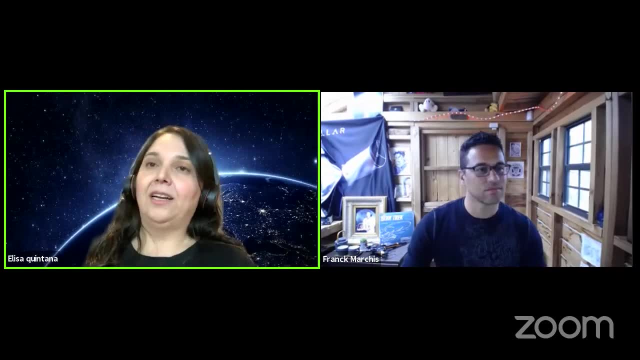 So we. so there are, you know, hundreds of planets already. you know would be great targets, So we so it's a one-year mission. We'll be doing data collection for a year. We can do an extended mission if we're successful and NASA gives us more money. 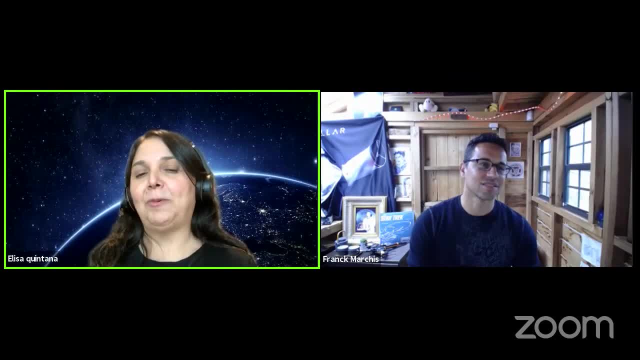 But it's a one-year mission And during that time- because we want to observe for a long time- we have a notional baseline of observing 20 stars with planets, And right now we made a notional target list. It includes planets as small as Trappist, so Earth-sized planets, and then it has Puffy and Neptune-sized planets. 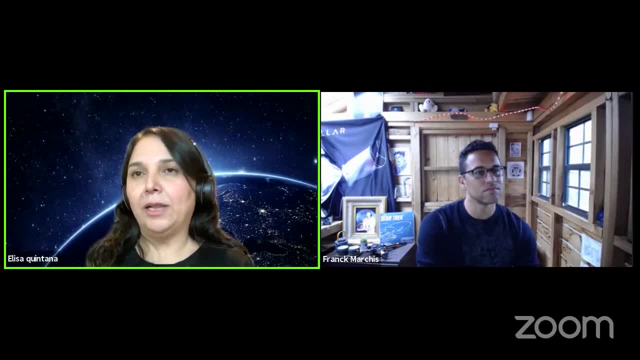 And the stars they orbit range from, you know, these small M dwarfs up to K dwarfs. So currently we're showing like, oh, we have these 20 planets. These are some good ones. A lot of them are already targets for James Webb. James Webb will be observing them. 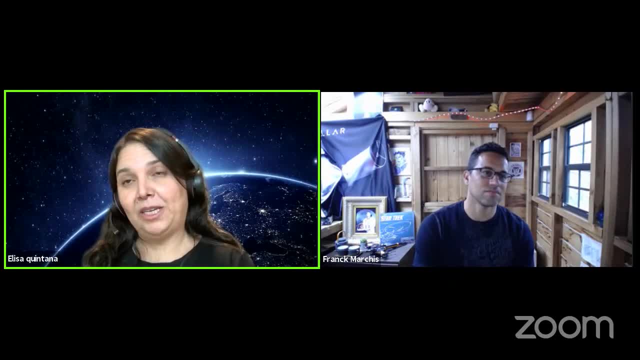 Pandora will be operating. So we can- you know we could monitor stars and planets at the same time, Or we can go back and revisit some of the ones that James Webb has looked at, But these are all changeable, You know we'll, we will learn a little bit. James Webb is going to launch this year. So by the time Pandora launches we'll have some information. You know they'll probably have observations of Trappist- everyone's favorite Earth-sized planets- And see if we can do that. They look good because you can instantly see if there's some signs of stellar contamination. 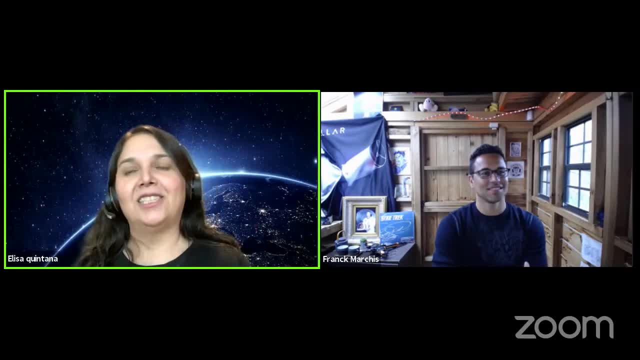 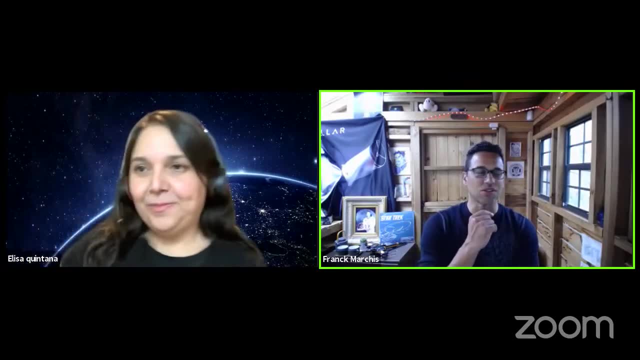 And so there's: yeah, we can swap in planets, you know whenever Good. We already have some questions And in fact, this is a question I wanted to ask you: What is the launch date for Pandora? What do you target? 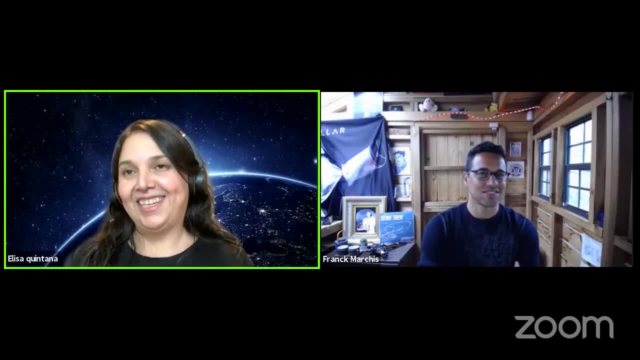 It's currently November 2024.. And yeah, so it has to be within the five years. So that's what we're aiming for. Do you have a vehicle or you don't know yet? It could be anything, Not right now. 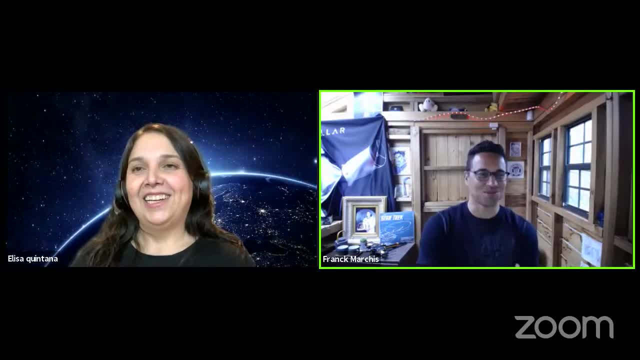 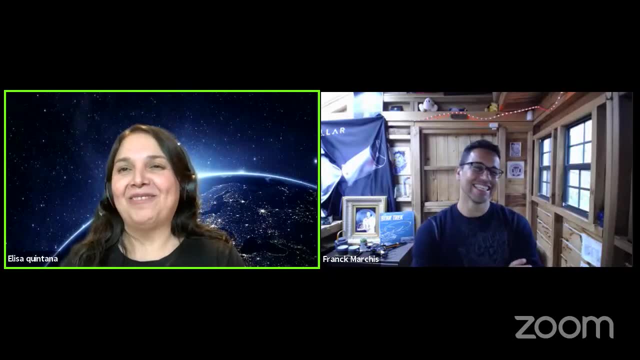 Not right now. Yeah, we have to still wait. So November 2024.. Oh my god, you're gonna be like stressed out in October. Well, I did attend the launches for Kepler and for TESS And I do remember watching the PIs for those missions. 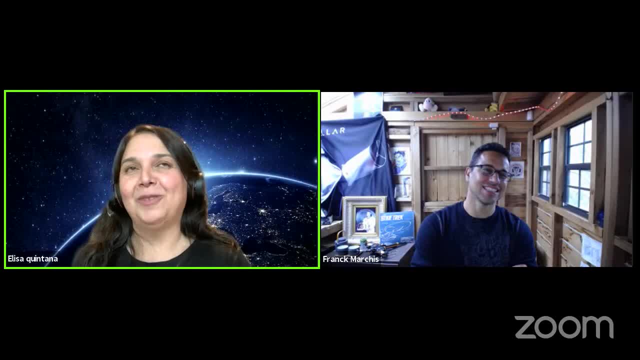 You know they well. actually, Bill Berucki, who was a PI for Kepler, was just cool. He's like it'll work or it won't. you know, he's like I'm pretty sure it'll work. 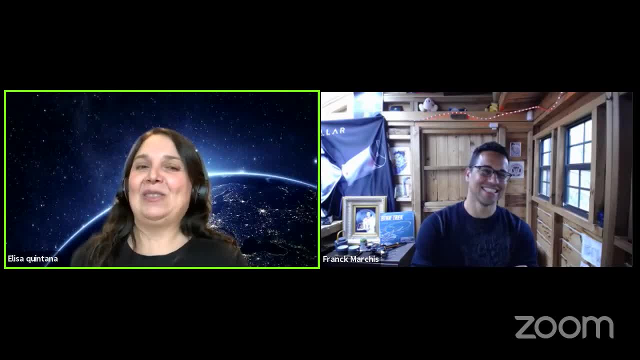 And he was like I'm pretty sure it'll work. And he was like I'm pretty sure it'll work. And then the PI of TESS was a little bit kind of nervous. But you know, they all went up successfully And they were happy. So you know. so you know, as I mentioned, small sets are riskier, but we'll cross our fingers. 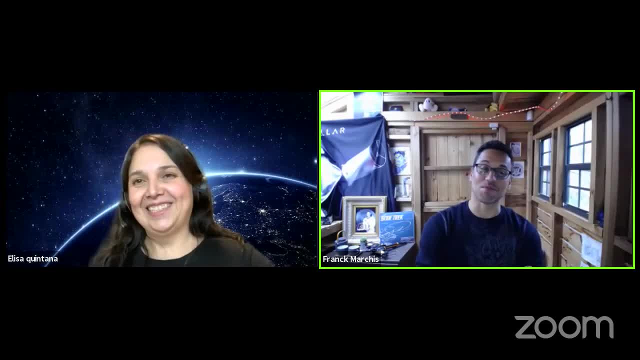 And hope for the best, Because if you don't take risks, you don't have rewards, right? That's the point of those missions. So you were at the launch pad. I didn't know that. You have seen a lot of launch of the key mission for the exploration of existence. 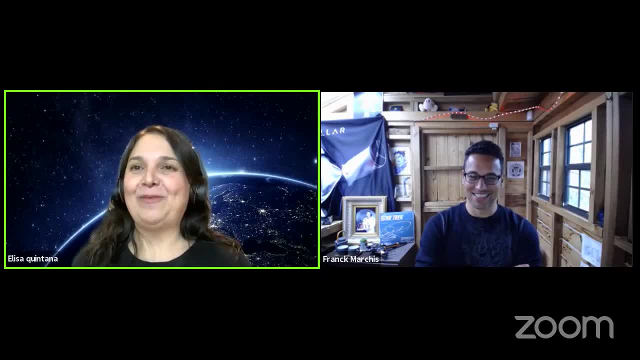 You know. so I was really impressed. I'm impressed. Yeah, Yeah, I was. I was lucky to be at NASA Ames when Kepler was being designed. That's still one of my favorite missions, you know. it's just so. everything that came out of it was just a surprise. 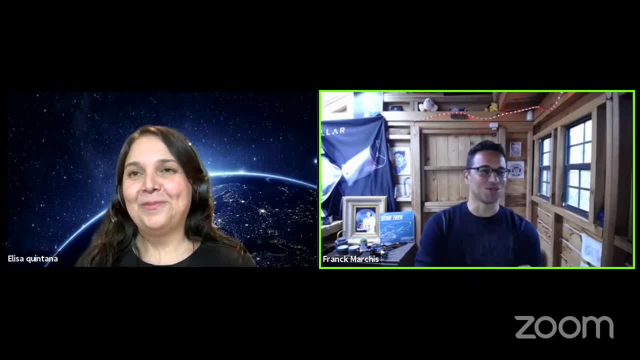 And it's a really fun mission to work on. Are you going to go to the JWST launch? I think it's in French Guiana or something, So I don't think many people are going, But I'll be watching very nervously, as a lot of people will. 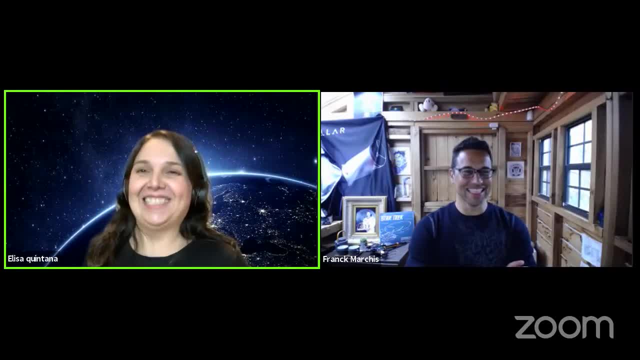 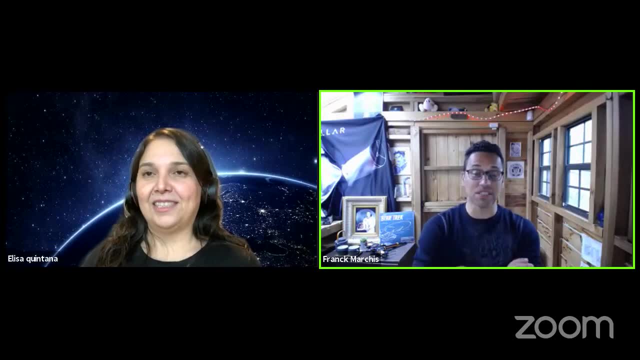 I will try to go there. if I could, That'd be nice. Yeah, that'd be nice. We have some questions here about the spectroscopic capabilities. You mentioned that. What is the range of the spectroscopic range of Pandora and maybe the resolution? 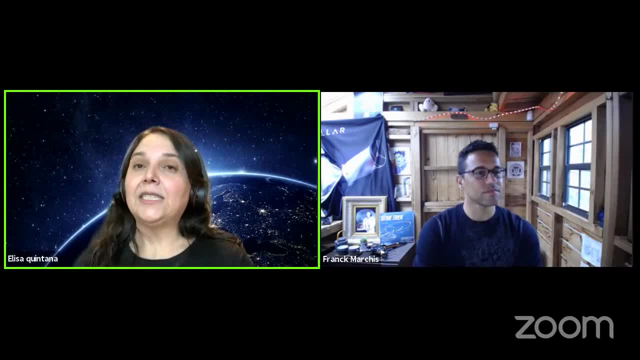 What do you expect to see in this area? Yeah, so we are still. we're in a phase right now where we're still trying to nail down Our everything, really our instrument. We- we do plan to use one of the spare flight detectors from James Webb. 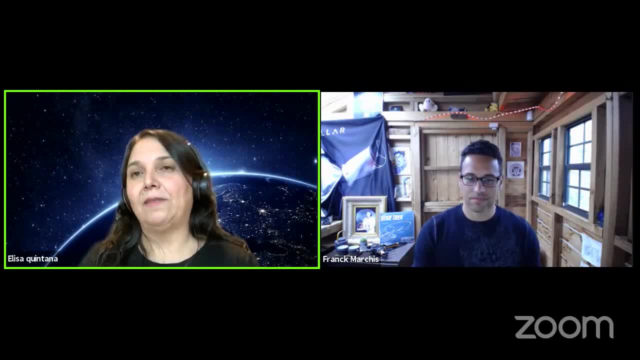 So after James Webb launches, then you know they have some flight that flight. These are these H2RG detectors for for the spectroscopy. We have a wavelength coverage that's comparable to Hubble's Wide Field Camera three And so. 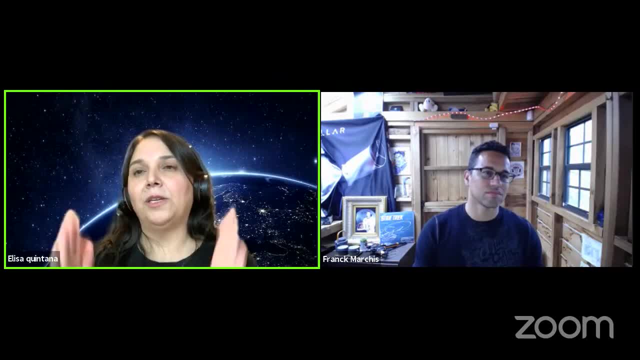 So something like, you know, it'll capture the water band, something like one to two micron, something like that, And the idea is really to correct for the stellar contamination and then, as a proof of concept, you know, look to see that we can observe water features And we 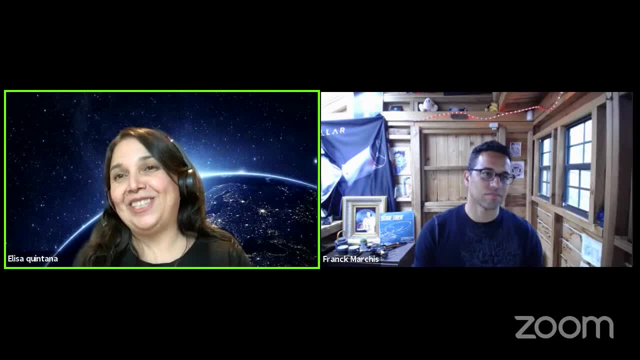 have some standard exoplanets where we know we see these features in Hubble, so we can double check that this works. And so it's kind of the two. first order. look at the atmospheres. Are they dominated by hydrogen? Do they have water features in their atmosphere, Are they? 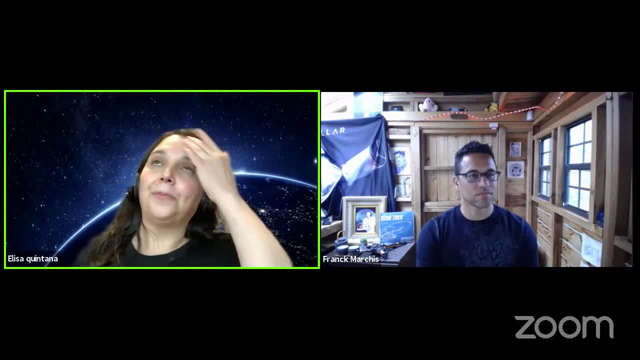 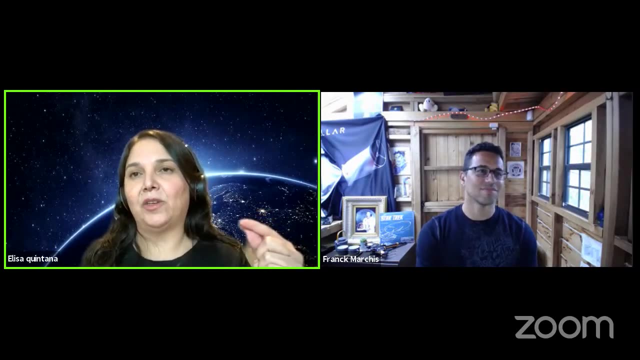 covered in clouds And you know a lot of the observations we've gotten for small planets have resulted in that And the you know a lot of results have said that. well, it looks like we have clouds because it's kind of a flat spectra, But what a lot of studies have shown recently is that stellar. 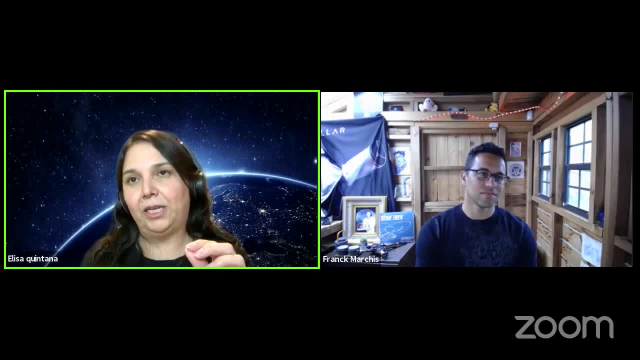 contamination. not only can it like mimic signatures in a planet's spectra, it can also suppress it. So there could be some exoplanets where they really do have some nice features, like a lot of these ones that we think are just cloudy- could actually have some nice. 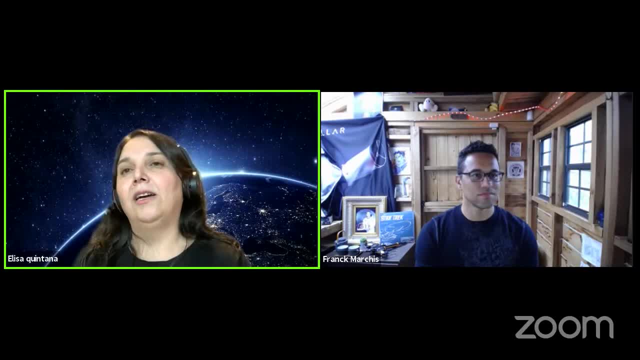 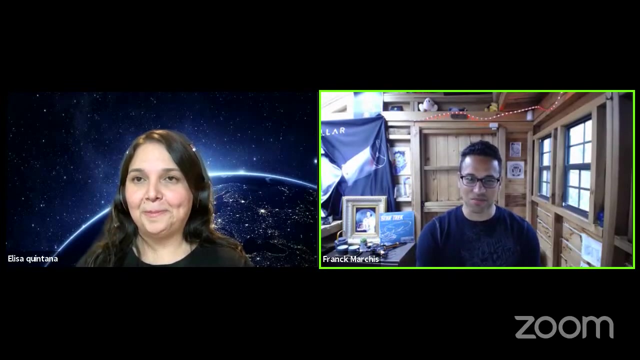 atmospheric features that are just being suppressed, And so so our goal is really to see what is the impact of this contamination and get a get a nice robust look at even those planets detected by Hubble or characterized by Hubble. We have people joining us from other places: Nish in Serbia and Fortaleza in Brazil, So 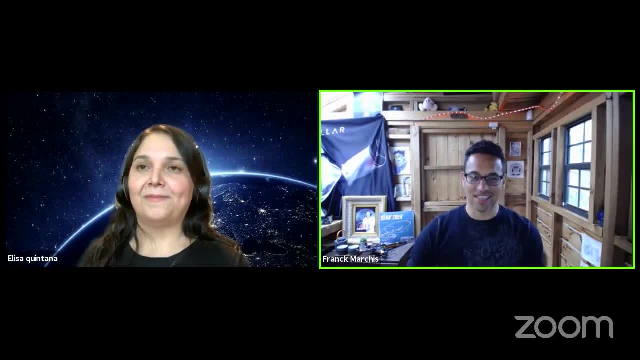 welcome And we're going to start with the Pandora small sat and this goal to characterize the atmosphere of exoplanets, planets in orbit around other stars. And I would like to mention to you watching us at the moment, that City Institute is a non-profit organization, So 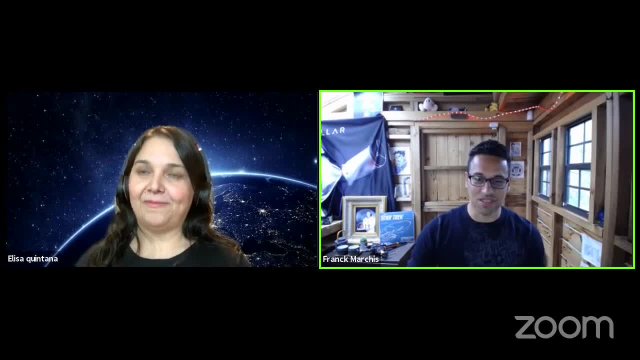 we appreciate your donation and we particularly appreciate the donation from Sabine, who sent us make a donation, made a donation on Facebook. So thank you very much, Sabine, And if you are French, merci beaucoup. Okay, So what else? So, oh, there is some questions about the satellite, small satellites, Everybody. 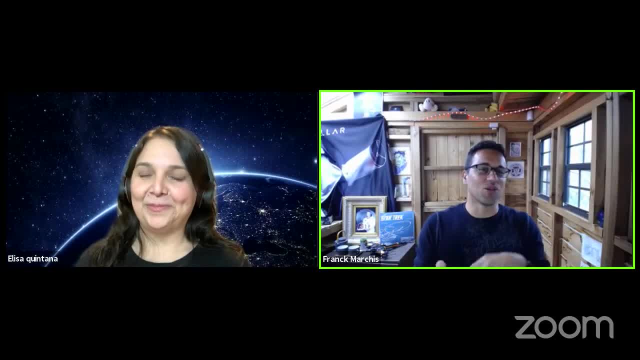 freaked out when you hear about small satellites, especially when they're in orbit around earth, which apparently is going to be the case for Pandora, right? What about the stability of the orbit, the pointing? Are you going? have you done some research already? with deliver. 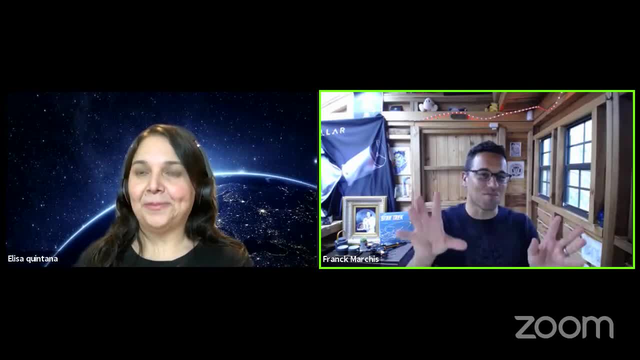 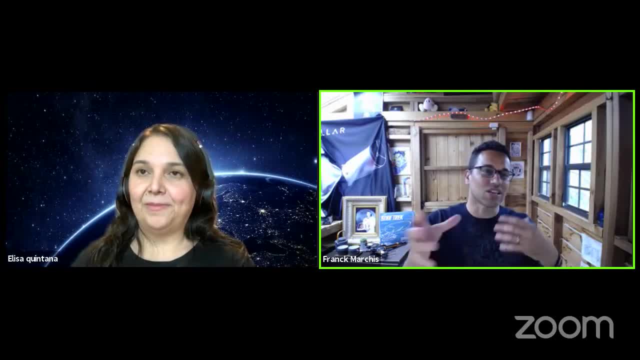 Yeah, Sure. So we would love to get those kinds of questions. if you have the technology to do this, we have the technology to compensate for those variations of temperate you when you all beat around the around the planet. So those are technical questions, engineering questions. 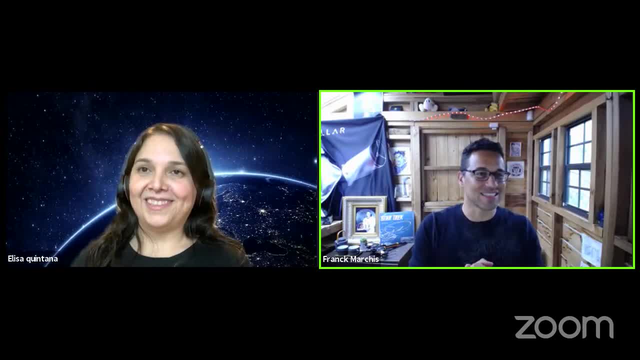 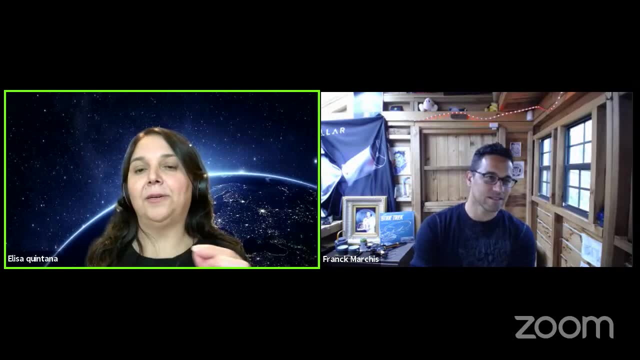 but it's an interesting question, So go ahead. Yeah, sure, So Pandora is going to be in a lowered orbit, But instead of going around you know the equator, it's going to be in a sun sink orbit. So what it is, it's kind. 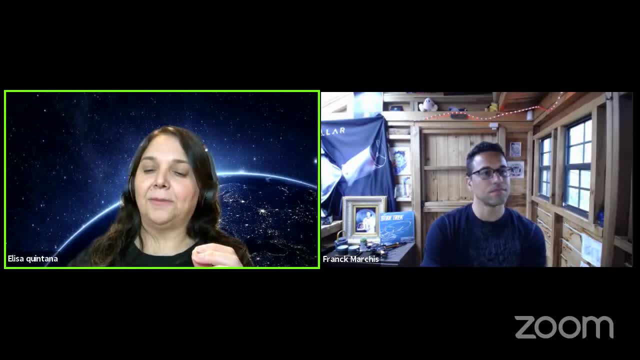 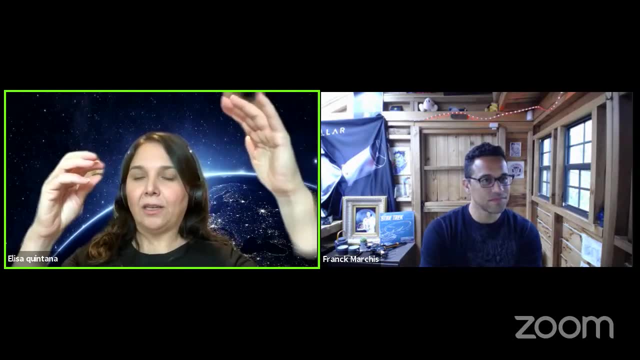 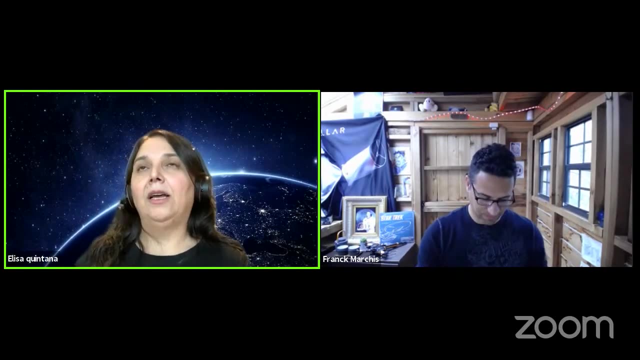 of going around. It's, let's say, sun sink lower orbit- Yeah, Sunsync, Low Earth Orbit, which will enable long stares at a really large portion of the sky, So we can observe exoplanets for a really long time. This is a nice orbit that you know. 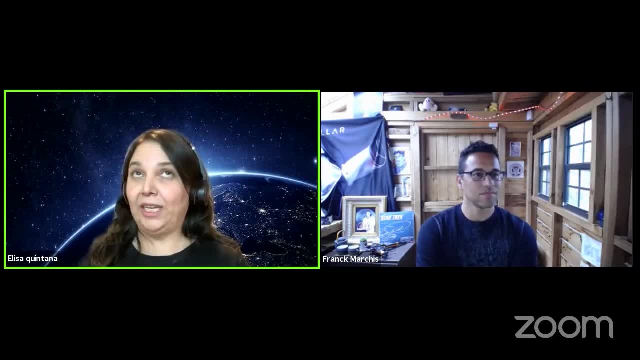 keeps us relatively thermally stable. We do need to have really good pointing, And so this is a common, you know, challenge for these smaller missions. There was another CubeSat called Asteria recently out of out of GPL And that was a small CubeSat And they were able to show that. 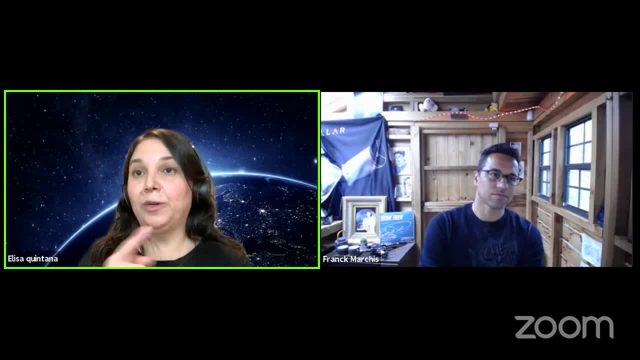 you can. using different techniques, you can get really good pointing sub-arc, second pointing on on some targets, And so we are kind of taking that knowledge and trying to work it with Pandora so we can get the pointing that we want the thermal requirements that we want. 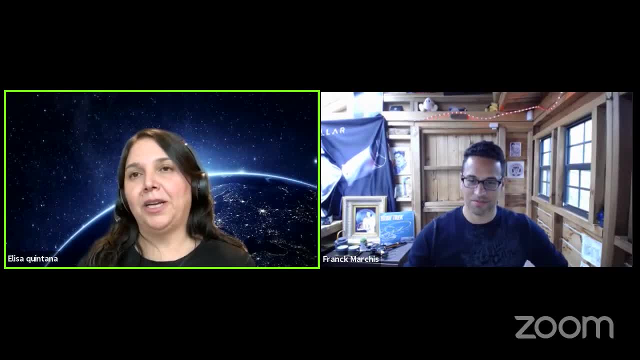 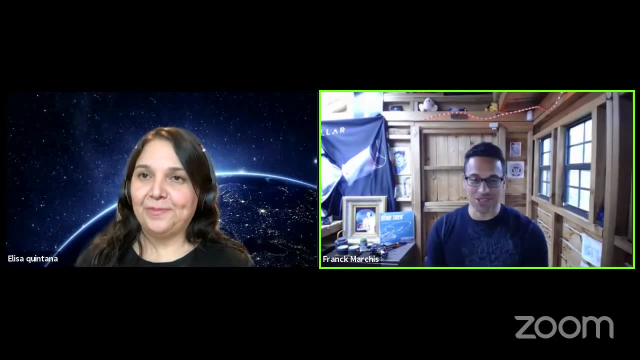 And it looks like we have a closed design right now. But yeah, those are all challenging, especially for these small, small missions that don't have a lot of mass Good. Some of the questions related to the data. So Pandora is going to take a lot of data. 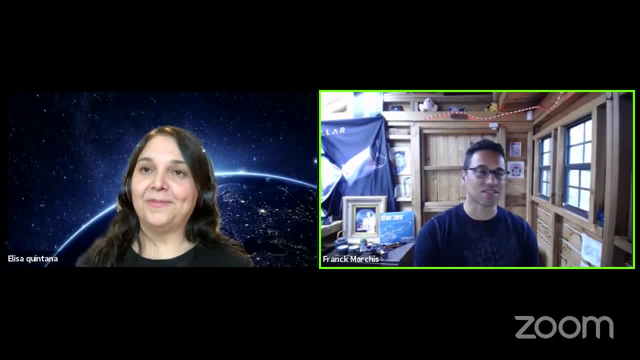 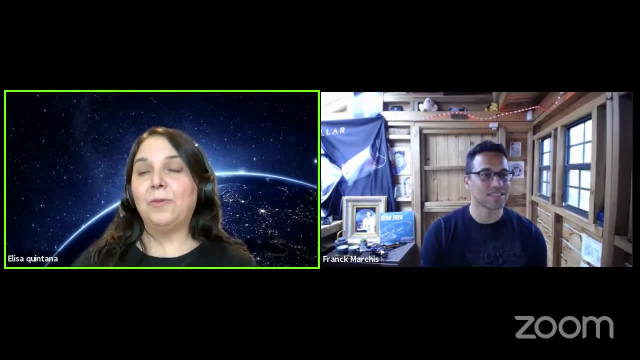 You mentioned like 100 hours of observation And then stars plus the transit of the exoplanets. Will this data be released and available to the public? Do you have a citizen scientist project linked to this Pandora mission? Yeah, so we have some people working on a data pipeline at NASA Ames, So these are. 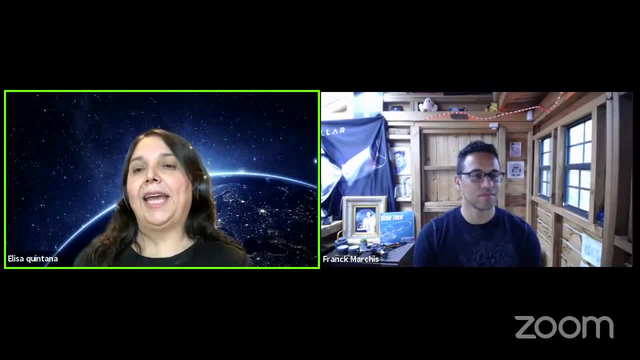 a group of people that worked on the Kepler and K2 missions, And so they are writing processing pipelines so that we can provide not just raw data but some light curves and, some time, varying spectroscopy and everything, And we are releasing it as soon as possible. 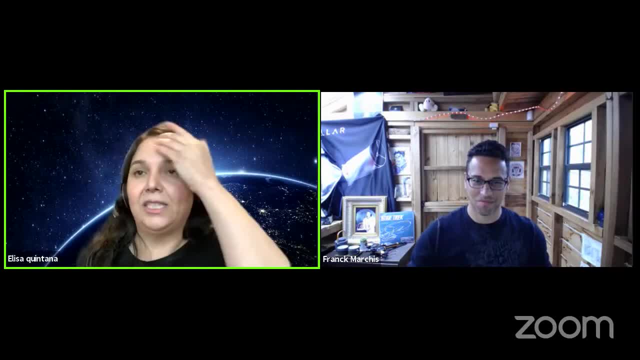 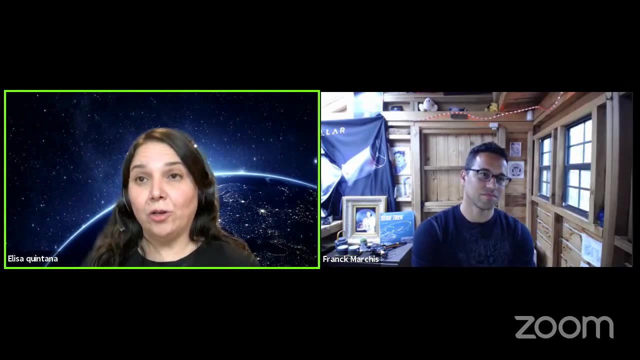 We want everyone to be able to take advantage of what we collect. So these small sub-programs don't typically have guest observer programs or participating scientists programs. But our project scientist is Nicole. She's the head of the project. She's also is Nicole Colon. She's also working on the James Webb Space Telescope, So she is going to put. 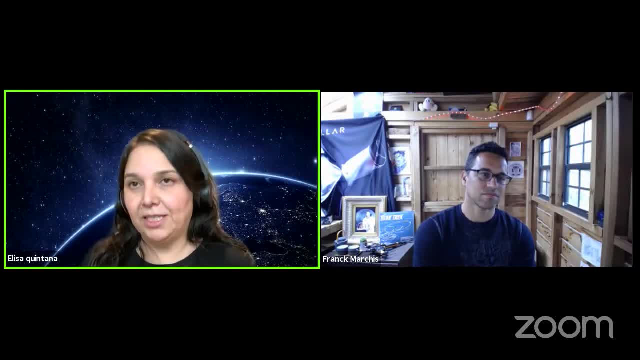 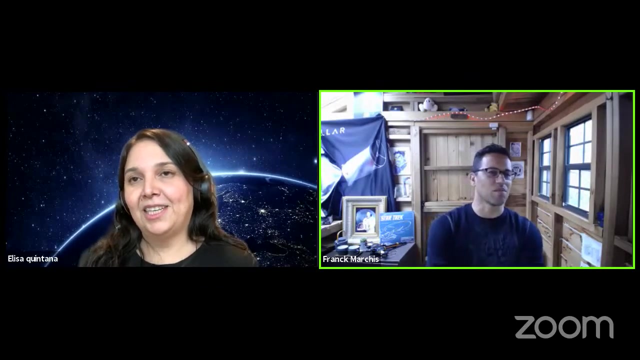 together a program to see how we can engage the community. We also are really excited about the opportunities for ground-based and other facilities to do simultaneous observations with Pandora. So there's a lot of opportunities for community involvement and so that we should be fleshing out sometime next year. All right, Do you have a website where you describe all of this? 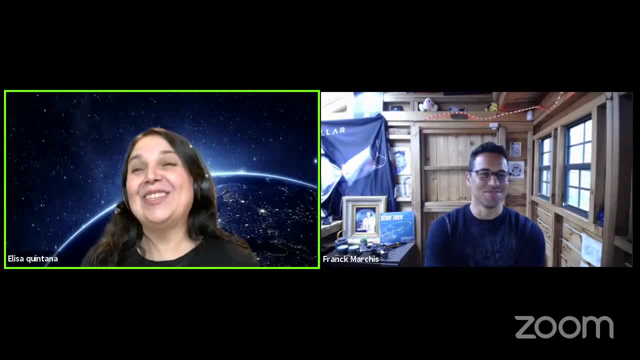 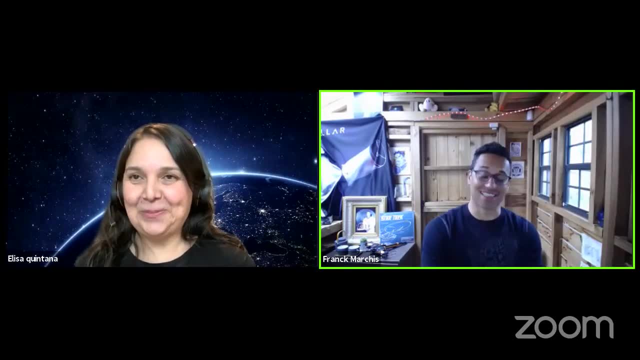 I have one in prep. I will do, yeah, Soon. yeah, We will post it and it's going to be already in the description. Okay, that'd be fantastic, Don't worry. All right, so one question that I mentioned to you briefly before we start. What's his name? Why Pandora? Because you opened. 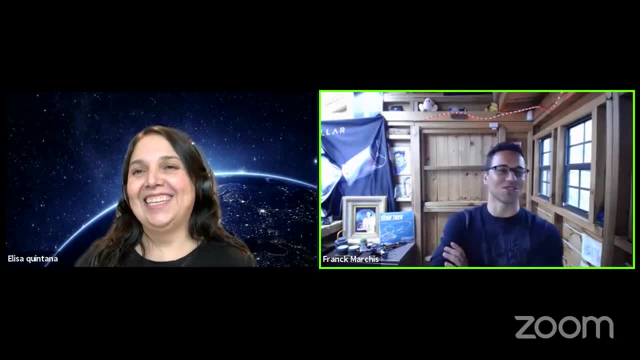 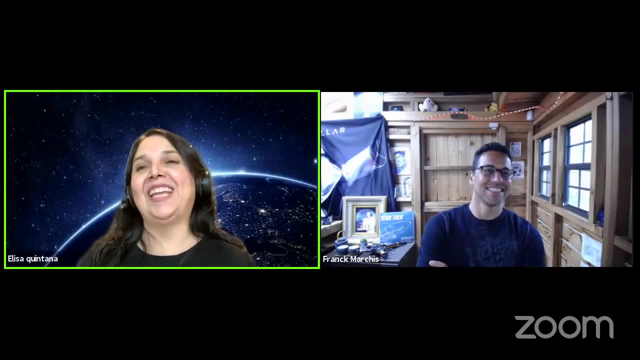 Pandora box. Why did we choose this name and who chose it? So it was when. so Pandora did start out as a CubeSat and it ended up getting bigger because we realized we couldn't fit everything in a smaller, in a small CubeSat. So I think 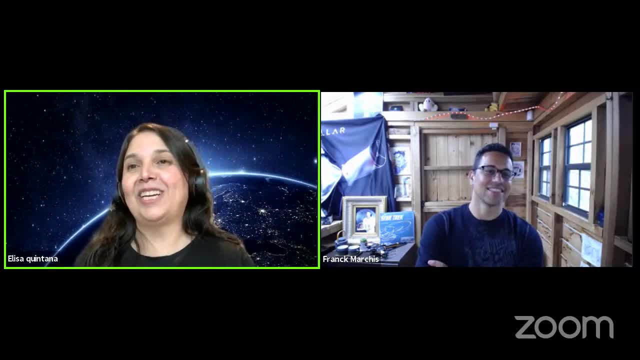 talking with Tom Barclay. he's an astronomer also working on TESS. He's an instrument scientist for Pandora. We were trying, we had to think of a name because we had to submit I don't know some paperwork And then we were like: what's it? we were thinking CubeSat and we're like: what's a box? 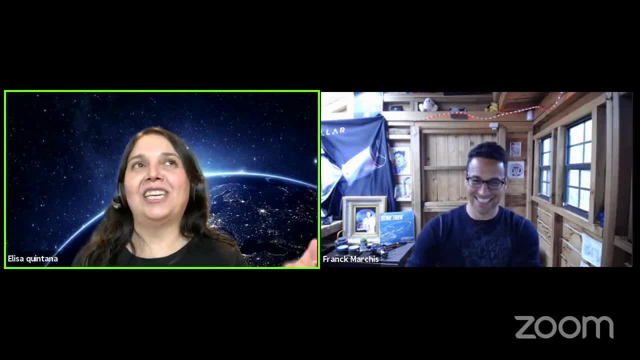 And we're just like Pandora's box. And then it was like a minute conversation And we're like, well, you know, it does have like earth and fire, you know like planets and stars, And so we just stuck with that And that's about as much thought that we put into it. We didn't want to do acronyms. 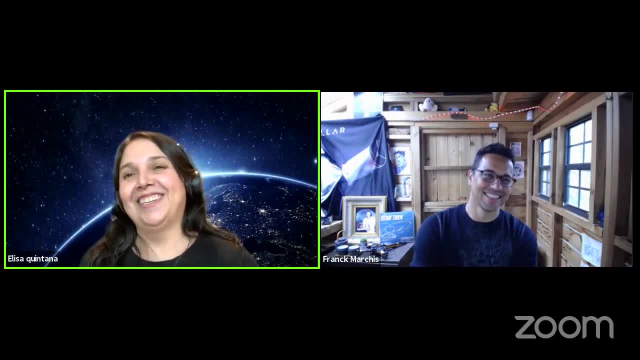 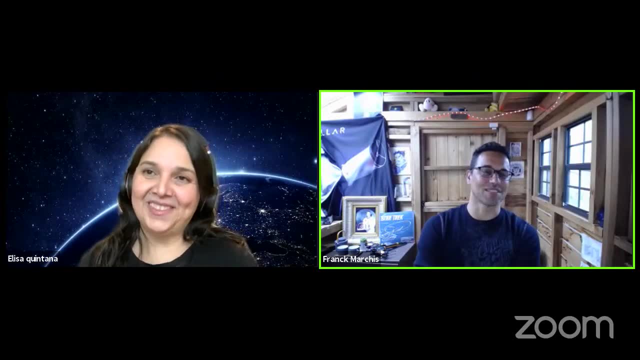 because we're trying to avoid acronyms And so it just kind of stuck. So nothing too deep. It's good to find a name like this. Really, names are found by having a conversation in the old way of a friend or scientist, or having two or three drinks in a bar. That's the best time to find. 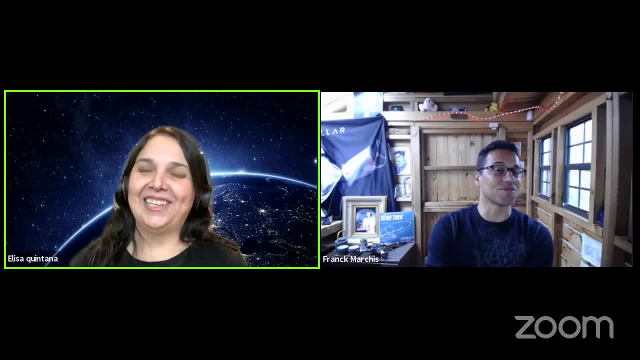 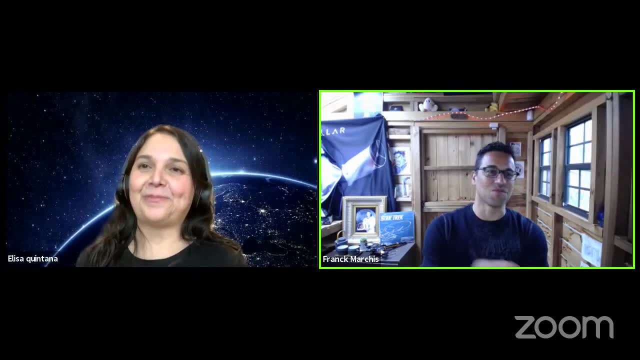 names for a mission And I'm very. I applaud the fact that you didn't want an acronym, because I'm also like people, my generation, we are the same generation. We are so tired of those acronyms. So it's great And we're glad to have real names for missions at our state. 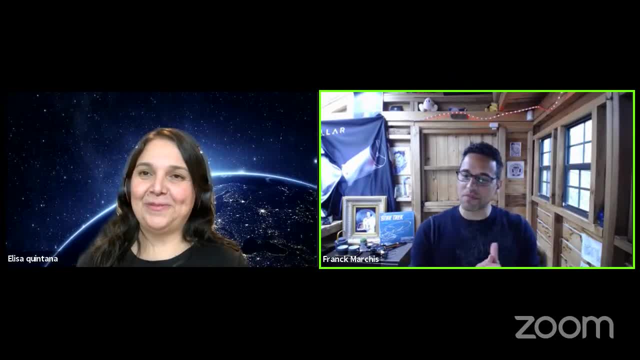 So, yeah, I think we're going to wrap up, but before we wrap up, I want to ask you about your life in the space. What's the next step for you? Are you the PI of this? Do you work on some something else, Or you dedicated full time on that? What's the 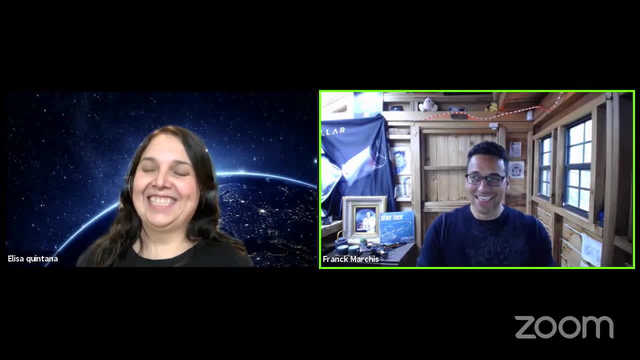 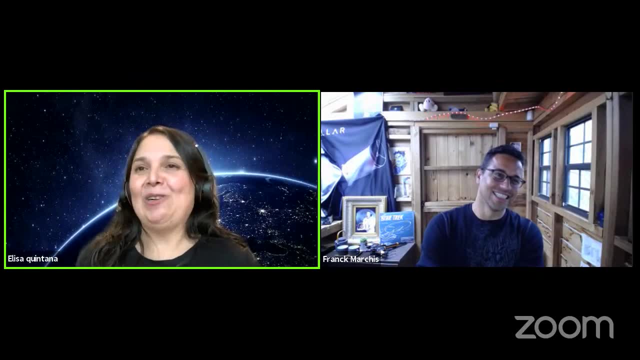 typical life of Elisa Quintana in Maryland. now, Yeah, so I've been at NASA Goddard for four years now. I'm currently deputy project scientist for the TESS mission. I've been working on communications for the Roman Space Telescope, but since Pandora was elected, I'm almost entirely. 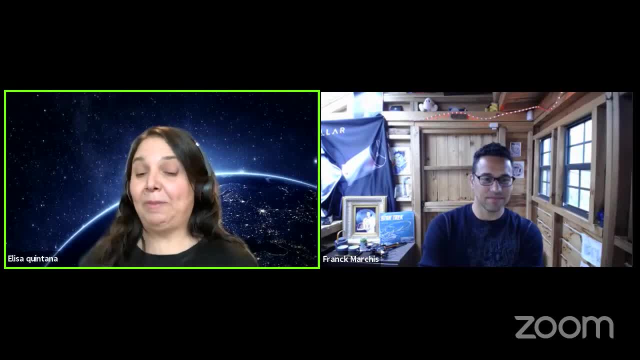 focusing on that. So what happens is we're in this initial period, we have to write up a report, NASA will give us a green light and then we'll be busy for five years. So I don't really know what's next. I've always wanted to. I did aerospace as a master's, in addition to my PhD in physics.